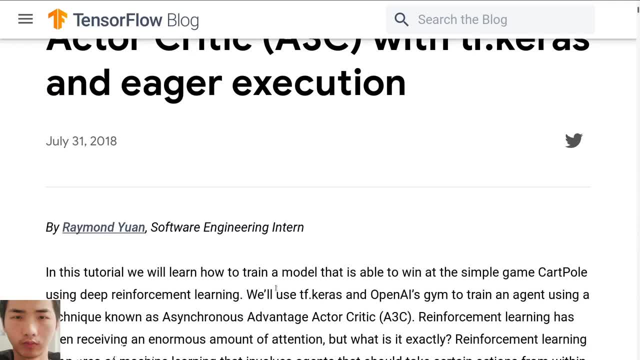 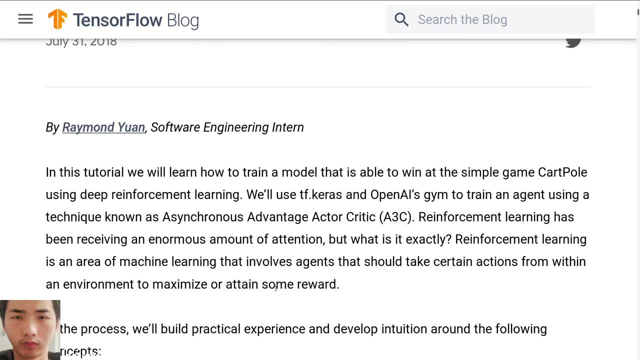 should be awesome. That would be awesome. Okay, let's get started. In this tutorial, we will learn how to train a model that is able to win at the simple game, CardPool, using deep reinforcement learning. We use tfcabras and OpenAI's gem to train our agent using a technique known as asynchronous. 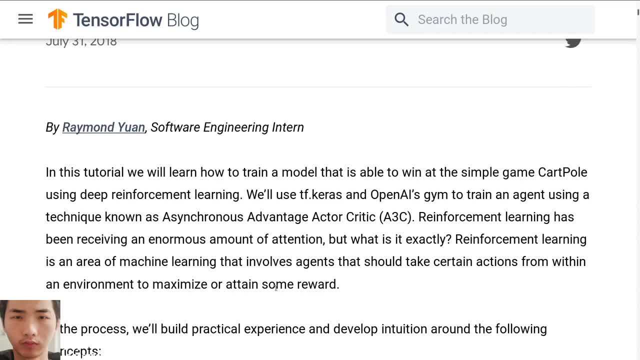 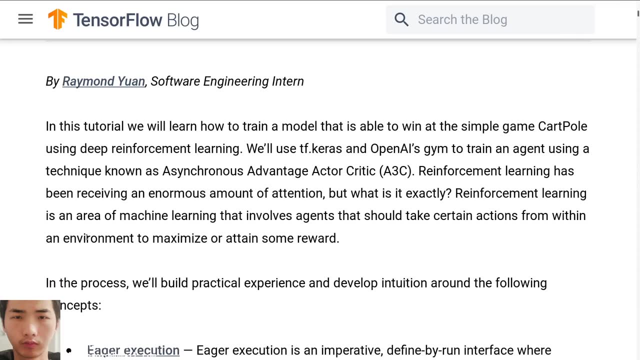 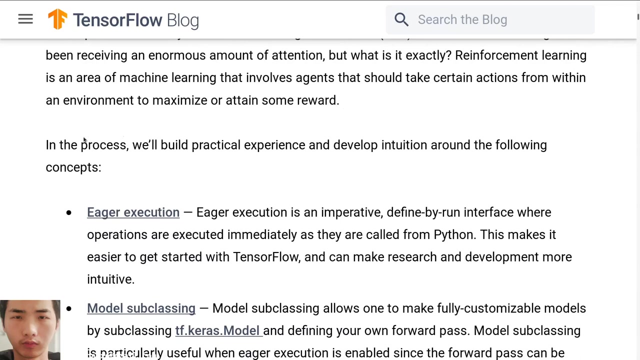 advantage actor critique. Reinforcement learning has been receiving an enormous amount of attention, but what is it exactly? Reinforcement learning is an area of machine learning that involves agents that should take certain actions from within an environment to maximize or attain some reward. In this process, we will build a process. 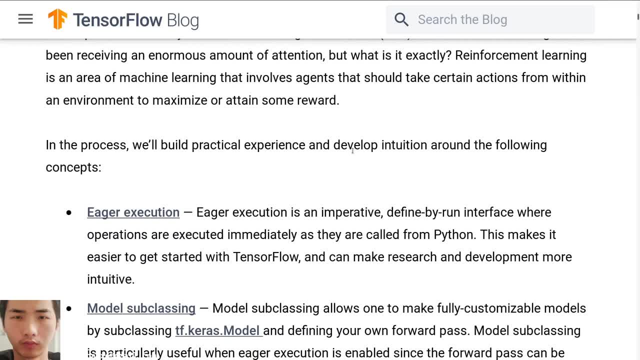 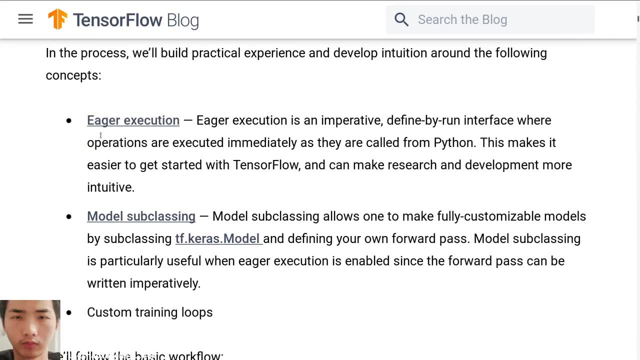 We will build a process. We will build a process, We will create a practical experience and develop intuition around the following concepts. The first one is the Agroexecution. Agroexecution is an imperative defined by Won interface, where operations are executed immediately as they are called from Python. 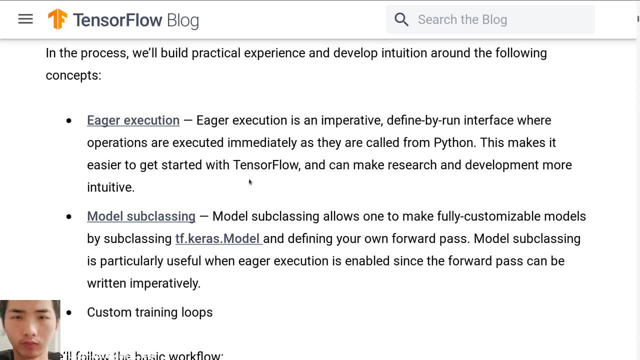 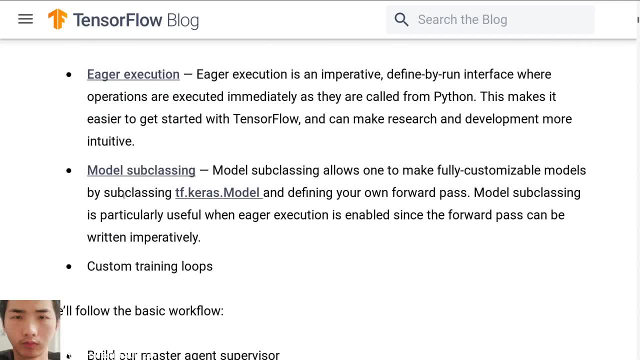 This makes it easier to get started with TensorFlow And it can make research very easy and development more intuitive. The second point is model subclassing. Model subclassing allows one to make fully customizable models by subclassing tfcarismodel and defining your own forward path Model. 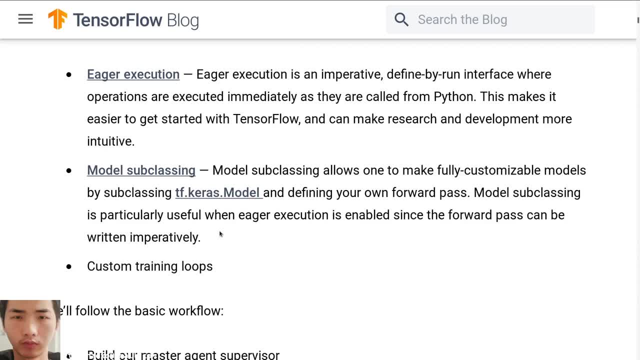 subclassing is particularly useful when error execution is enabled, since the forward path can be written imperatively. So here comes the concept: model subclassing In general. in my daily routine I won't use that technology. Instead, I'll use the sequential model or the API. 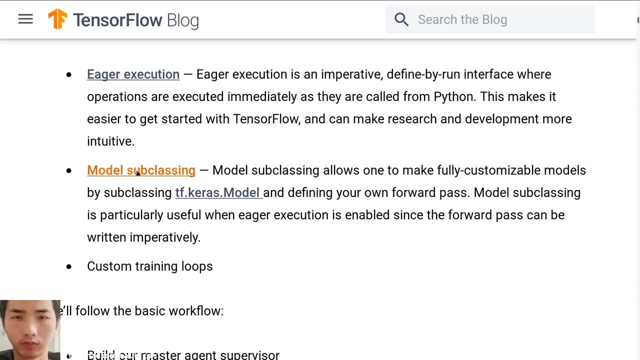 functions in Caris. I won't use this technique, But as far as I know, the PyTorch and Elnabry are based on class. You know, if you want to make a model in PyTorch, you can create a class. So this is a seminar with that. 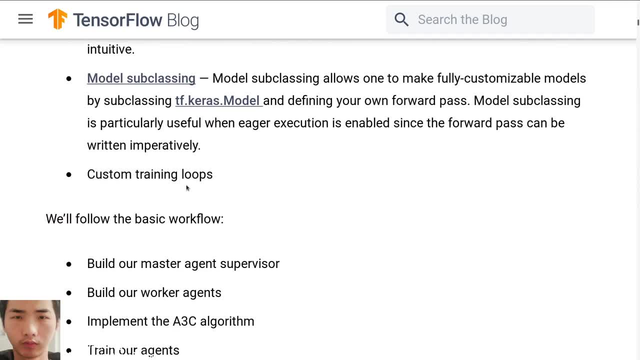 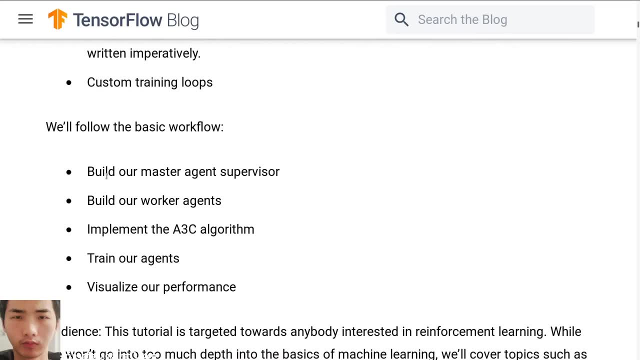 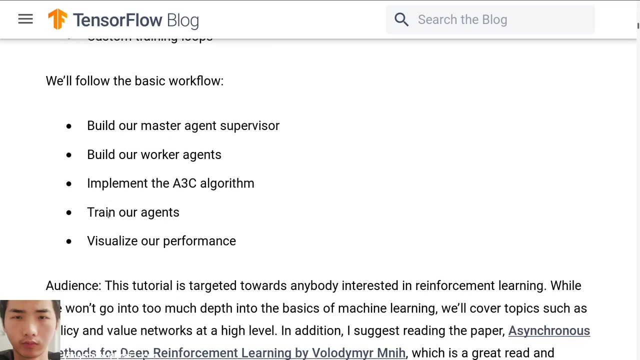 3. Custom training notes. We'll follow the basic workflow. Let's say, first we have to build our master agent supervisor. 2. We have to build our worker agents. 3. We have to implement the a3c algorithm. 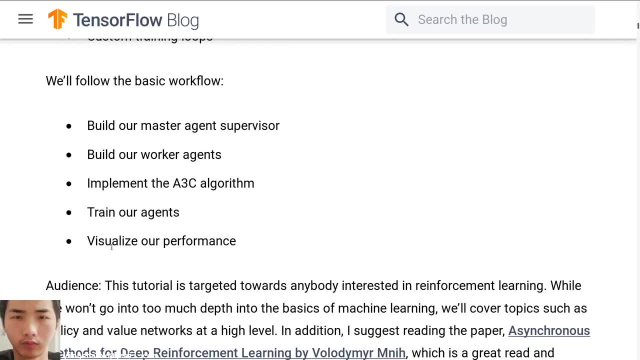 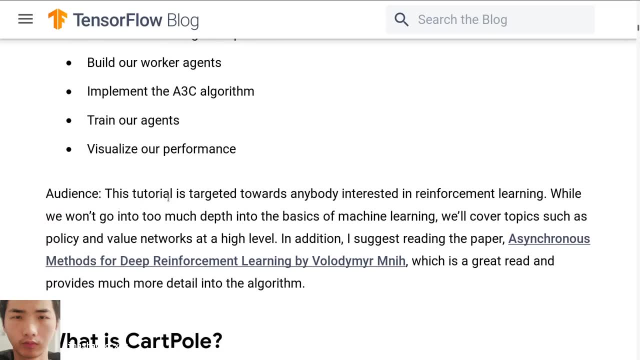 4. We have to train our agents. 5. We have to visualize our performance Aliens. This tutorial is targeted to update user experience and performance for all customers in the company. This tutorial is targeted to improve the performance and performance of the colleague. Don't forget to click the subscribe button. 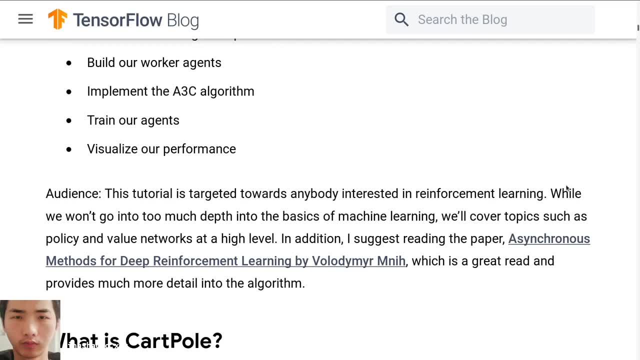 towards anybody interested in reinforcement learning. while we won't go into too much deeps into the basics of machine learning, we'll cover topics such as the policy and value networks at a high level. in addition, i suggest reading the paper i sync rose: methods for deep reinforcement. 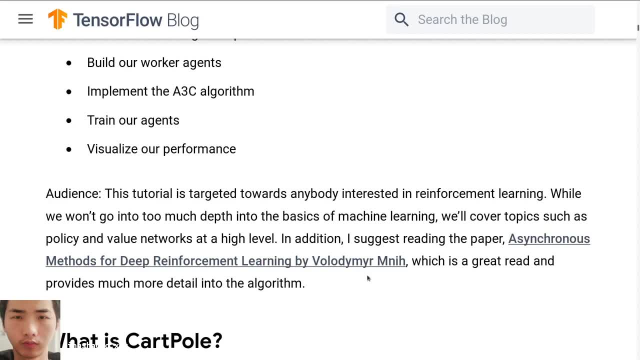 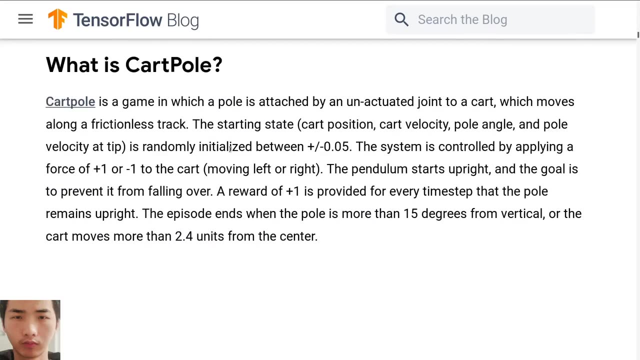 learning by. i don't know how to read that, but it's a. it's a person name, which is a great read and provides much more detail into the algorithm. what is carpool? carpool is a game. yeah, literally it's a game. it's a very simple game. 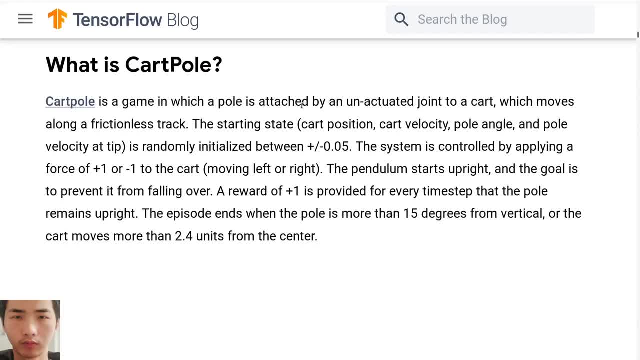 in which a pole is attached by an arm actuated joint to our, to a card which moves along a frictionless track. the starting state: the card position. position: card velocity: poor anger, polar anger and polar velocity. a type is readily initialized between negative 0.05 to positive 0.05. the system is controlled. 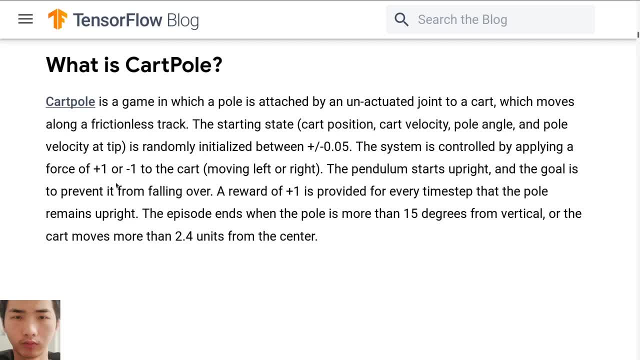 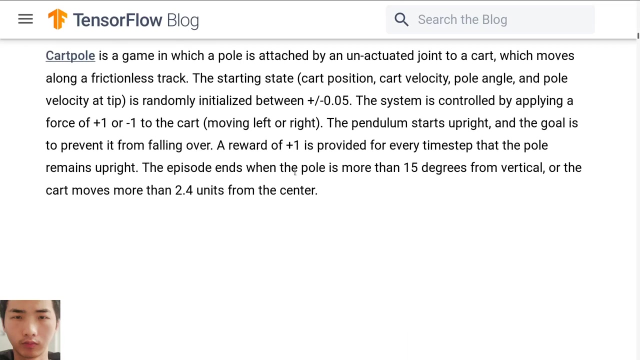 by applying a force of positive one or negative one to the card, moving left or right. the pendulum starts upright and the goal is to prevent it from falling over. a reward of positive one is provided for every time step that the pole remains upright. the episode ends when the pole is more than 15 degrees from vertical or the card moves more than. 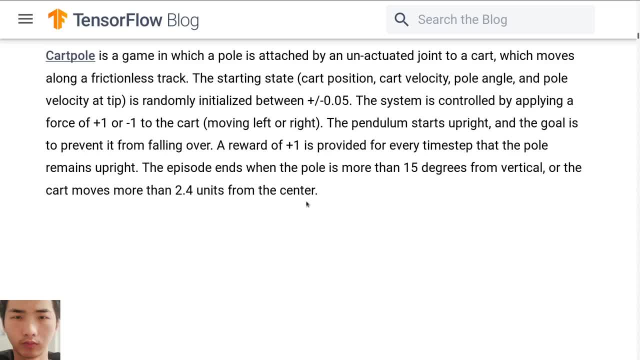 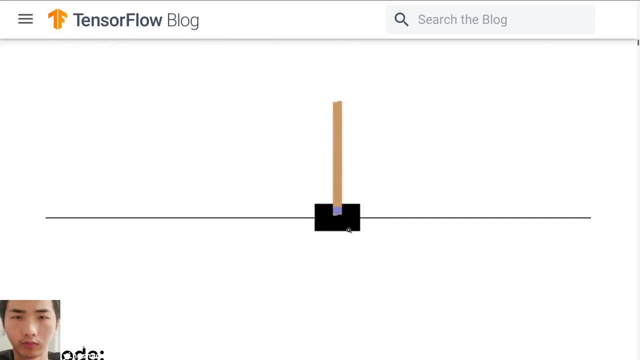 2.4 unites from the center. here is the general example about how this game looks like and, as you can see, here's a vertical line. it's not a vertical line, it's a. it's a ball, right, i, i guess? no, it's not a ball, it's a. yeah, you can think it as a vertical line for this line. um, it will fall down. 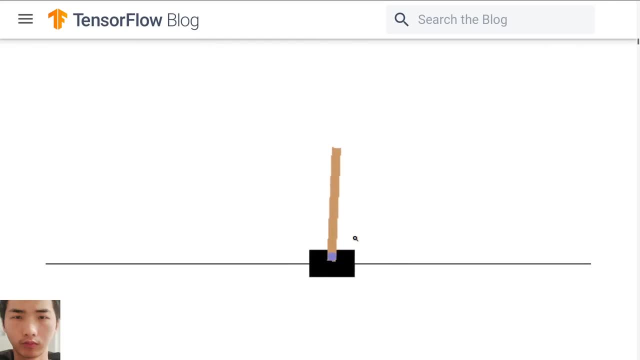 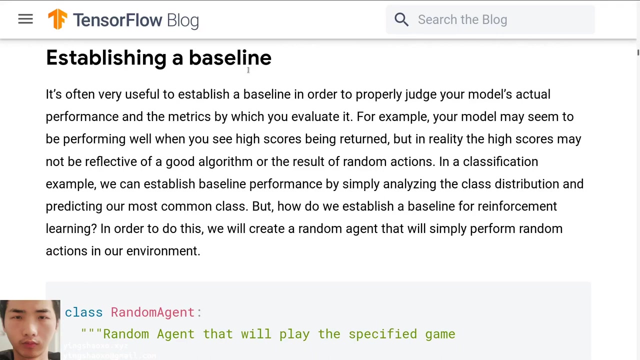 just imagine if you put your pen right on the desk. when you leave it alone, it will fall an arm and all mission is to light this vertical line. keep straight. vertically establishing a baseline. it's often very useful to establish a baseline in order to properly judge your models, actually. 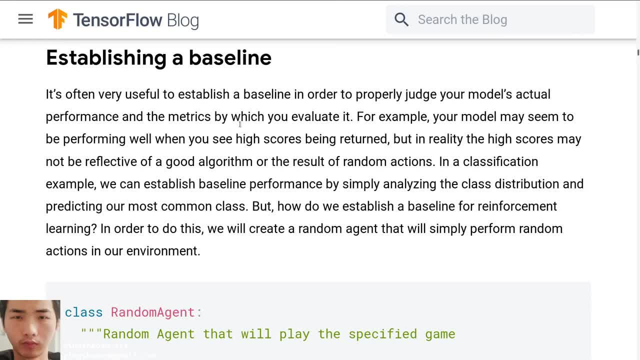 performance and the matrices by which you evaluate it. For example, your model may seem to be performing well when you see high scores being returned, but in reality, the high scores may not be reflective of a good algorithm or the result of written actions. In a classification example, we can establish: 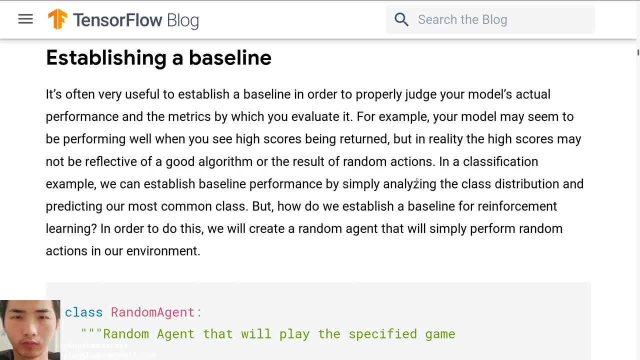 baseline performance by simply analyzing the class distribution and predicting our most common class. But how do we establish a baseline for reinforcement learning? In order to do that, we will create a written agent and will simply perform written actions in our environment. Okay, before we take a look at the code, let us think about this. 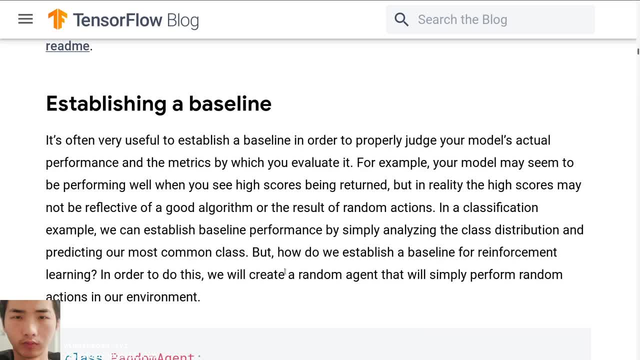 How can you say you are intelligent? The simplest way is to compare you with a written action. people, The written actions does not have logic inside of it, but you do sense based on logic. So that's the difference and that's why you should be aware of it. 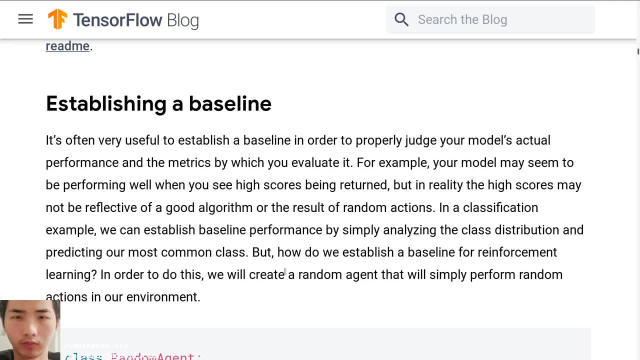 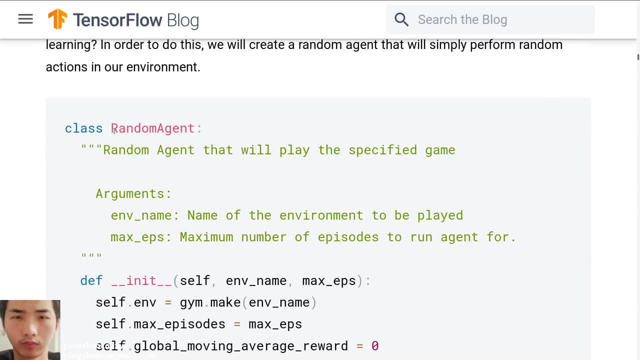 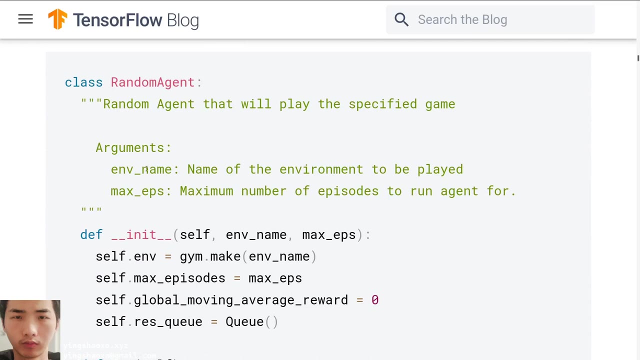 You have the intelligence, while the written mind doesn't. Here we can see he just created a class which named the written agent. This written agent will play the specified game. In here is a car polo. The argument is in weapon: the lamb lamb of the environment. 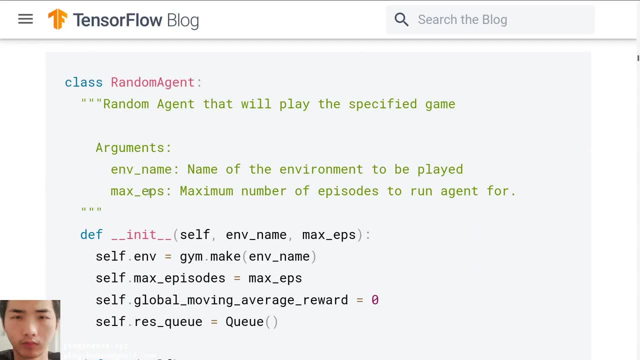 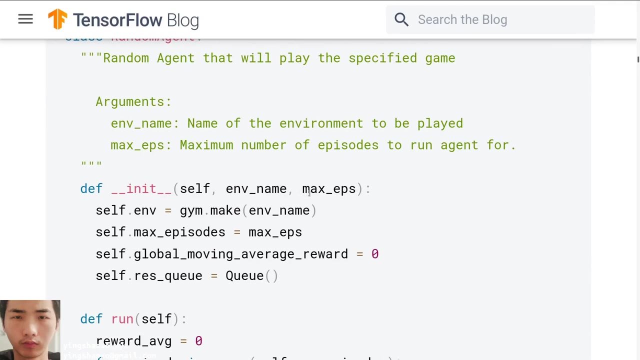 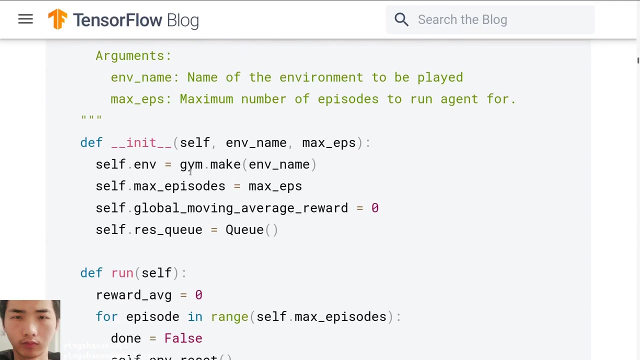 To be played on the maxed epics. maximum number of episodes to run. the agent for the initial function is the two arguments: the environment, land and is a maxed episodes. the environment equal to G, Y, M, GM that make the environment land the method episodes equal to the maxed episodes. the global moving average reward equal to 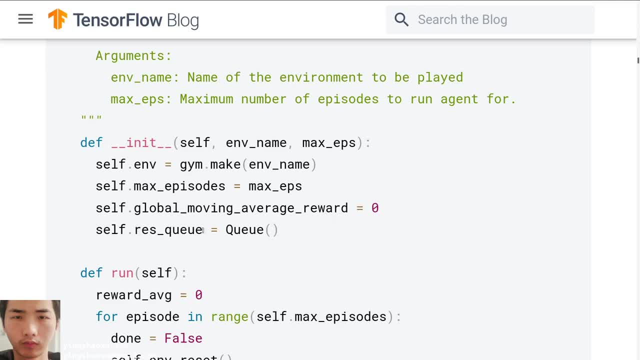 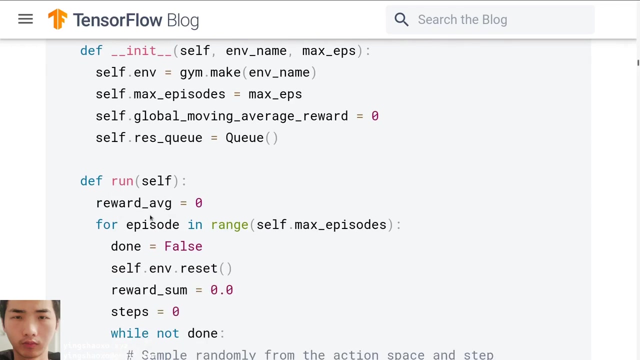 zero, the RAS cream equal to cream. no, we have to call it Q. yeah, what is Q in Python or in general ideas? Q is a data structure for representing data. let's say, first in first odds, that's a kill. then we have defined a function wrong. 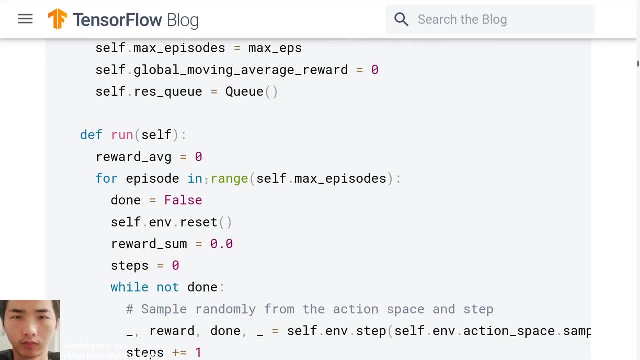 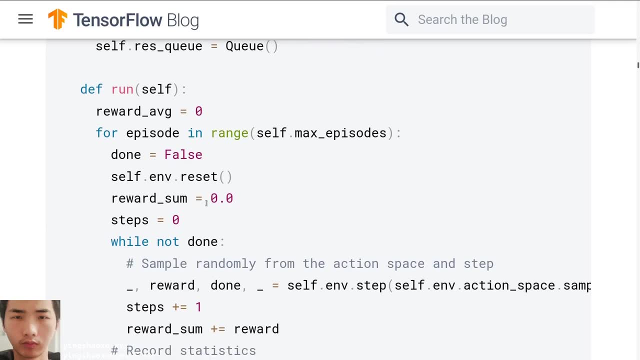 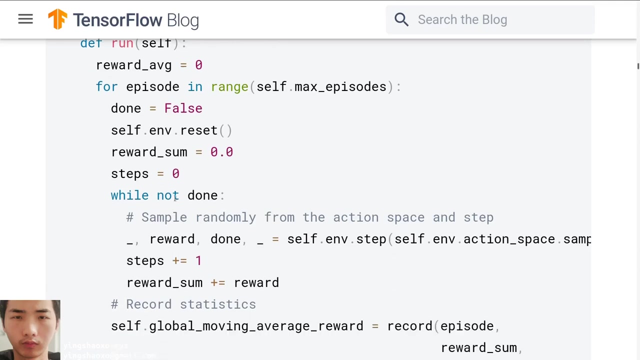 we wore average equal twoouch for episode in the range of maxe. the episodes don equal to force, save that in white man. to reset the reward song equal to seal. song of reward equal to zero. the steps equal to zero while not done in other, in another words, while this game is still on. 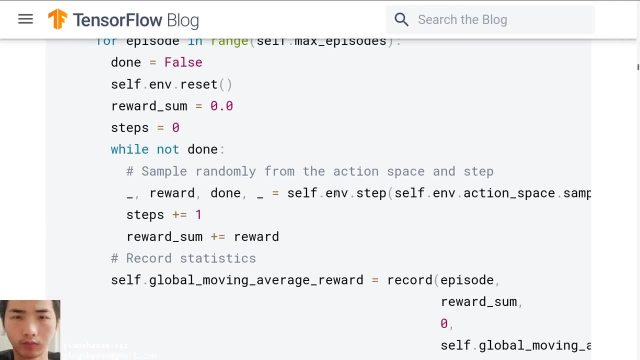 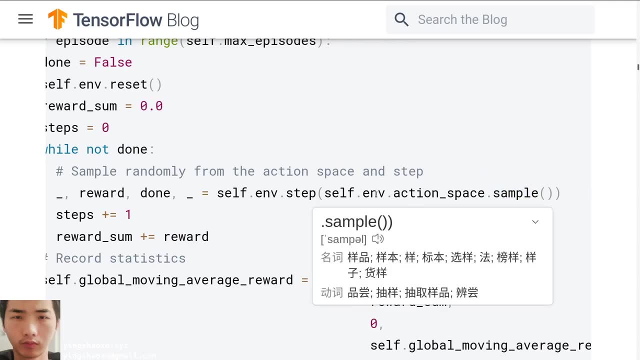 we do the following things. we do the environmentsteep, which means we have to take an action to the, to the environment, and this action is a reading one, as you can see here he just called environmentaction space. from the action base, we take a reading one using 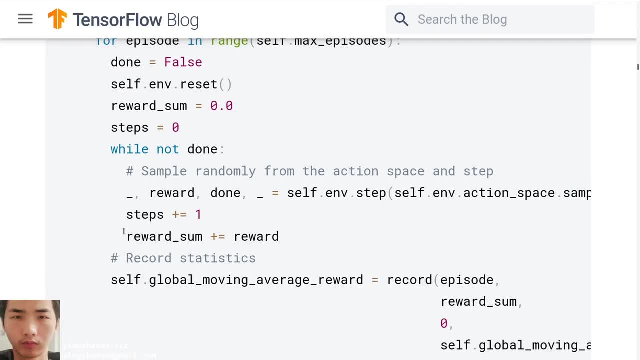 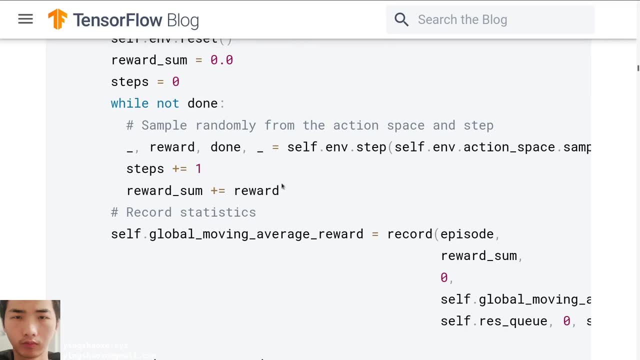 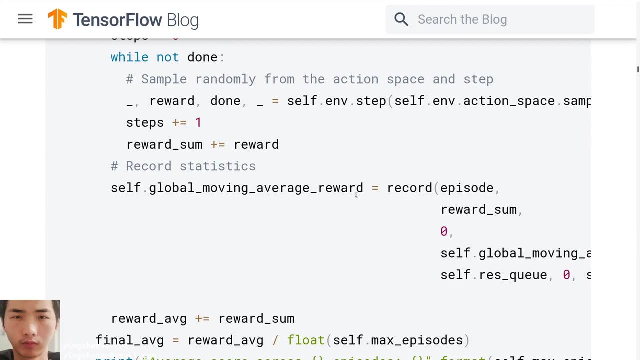 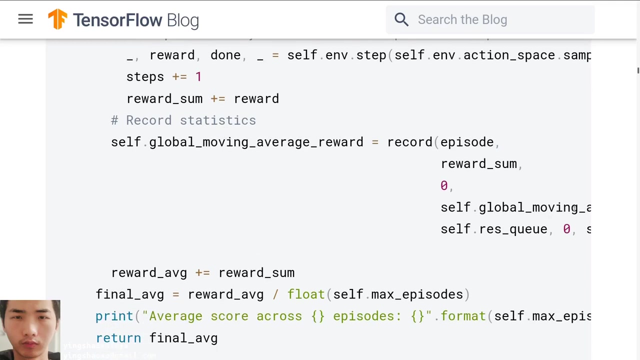 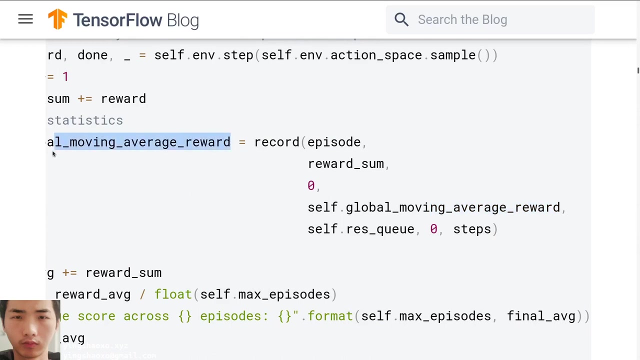 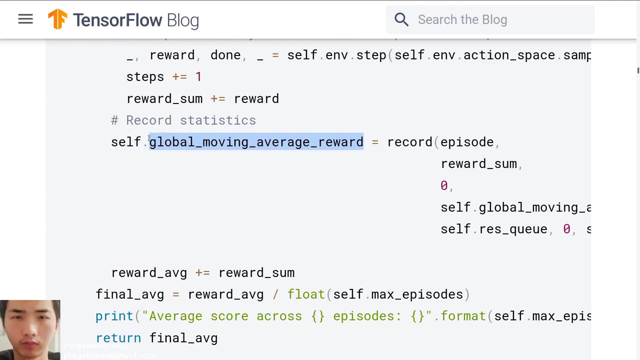 a sample function, then steps plus one: the reward song plus the reward record statistics: selfglobal moving average reward equal to the record episode reward song. zero global moving average reward and all those things. i don't know what's that mean, because i haven't. i didn't use it in my project before this, before this reading. 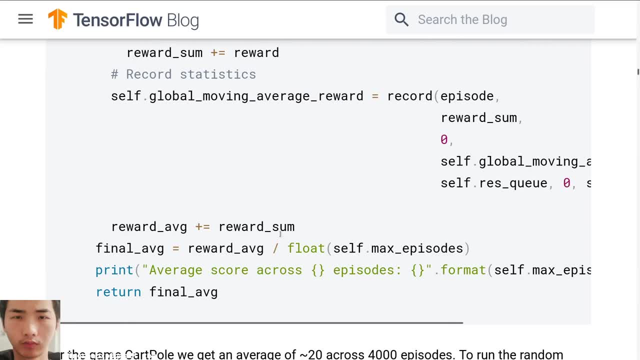 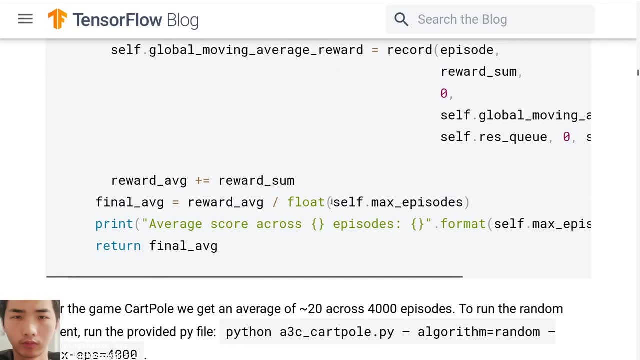 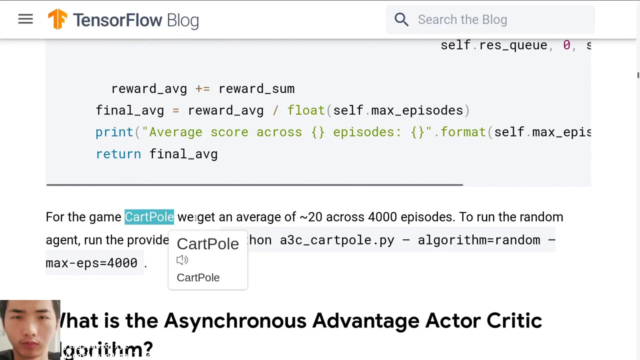 the reward average equal to the reward song plus a reward song, and in the end we have to divide it by the maxed expose so we can get the final average reward. for the game called polo card pro, we get an average of 20 across 4 000 episodes. 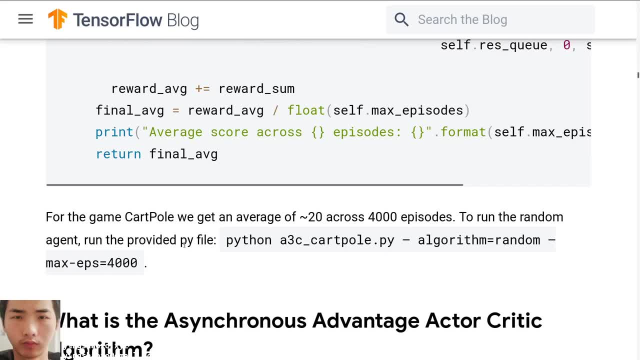 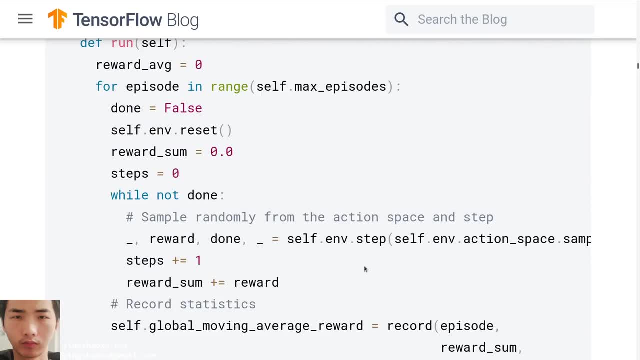 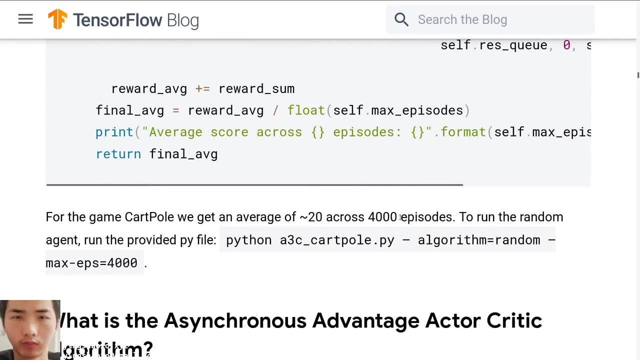 to run the reading agent in the provided py file. okay, that's it. that means, if we take, if we run this game four thousand times, let's say it will die four thousand times- and we will get almost 20 average rewards in that game. so for each game, for each game we will get. 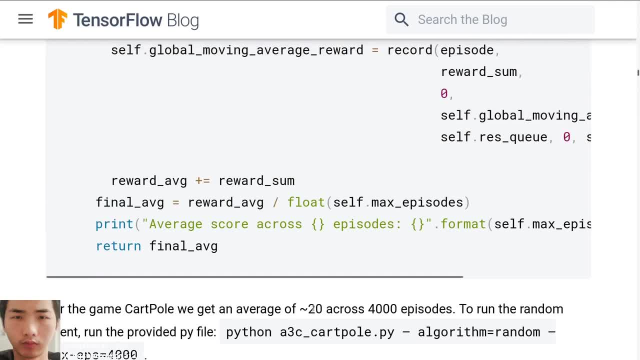 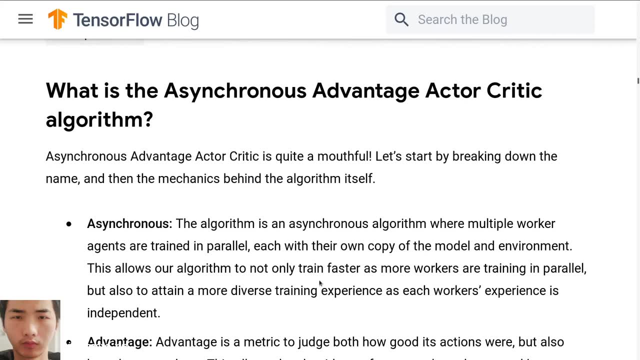 20 reward from that. this is an average reward. i guess you may ask me why i always recording videos on those stuff- i mean the machine learning. but it is very simple: because i cannot find any passion from other domains like the like the traditional programming. It's kind of weird for saying that, because I 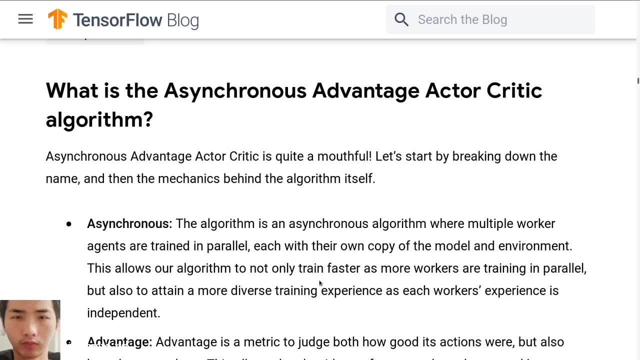 wasn't good at the algorithm side. I mean, if you want to be a good developer or a good programmer, you have to know a lot of useful algorithms, and clearly I wasn't a smart person, as you know, so I couldn't master those algorithms that much, so basically, I can't do that For me. the best way to overcome this is: 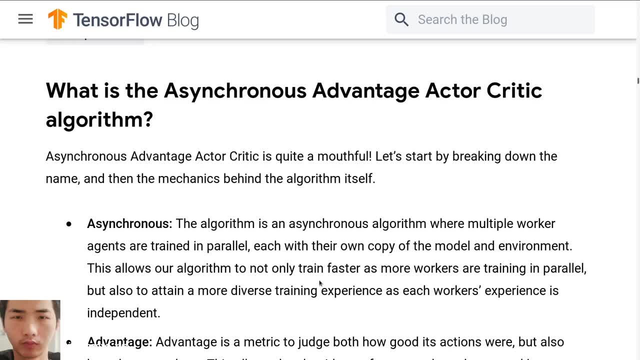 to find a new tool, a new strategy for us to get into complex the problem like the, the, the machine learning, machine learning. why machine learning is so outstanding? outstanding? well, it's simply because, um, for a problem, you can do it with the, the traditional algorithm, or, if you can't master that algorithm, you can train a neural network to generate, to generate. 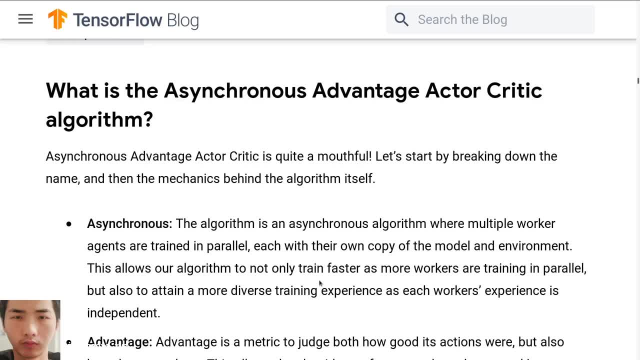 that algorithm. even this will take you a lot of computing uh resources, but it is worse for for you because you don't. you don't have to handle those complex equations by yourselves anymore. all you have to do is define a model and feed that model a lot of data and the 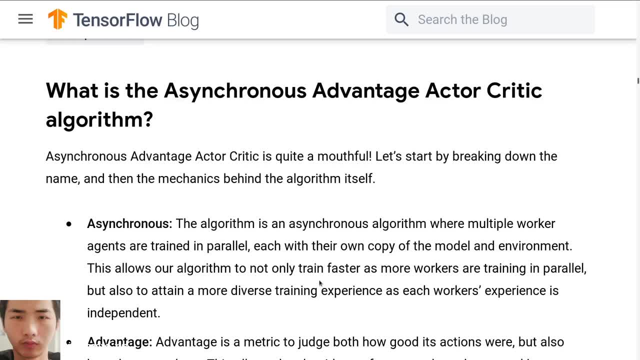 the neural network will will generate that algorithm for you. Okay, now let's get into the core part. What is the isynchro's advantage actor critic algorithm? Isynchro's advantage actor critic is quite a mouthful. Let's start by breaking down the land and then 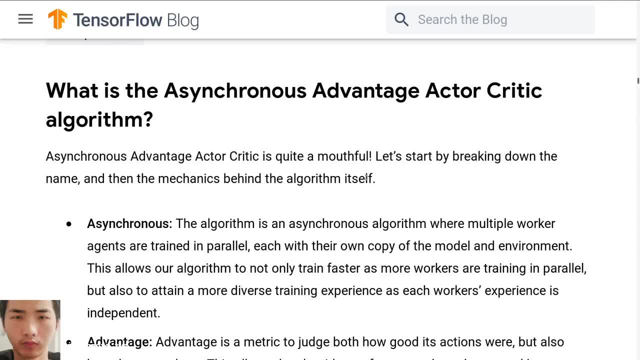 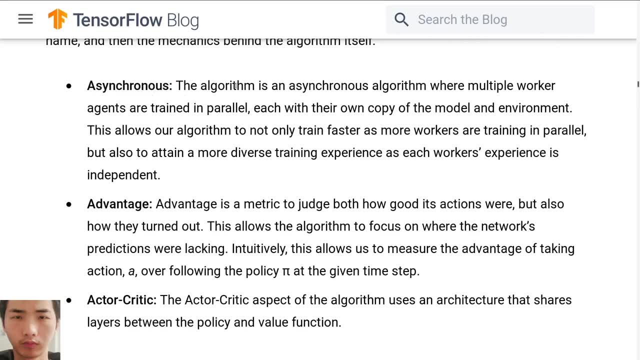 the machine leaks behind the algorithm itself. Isynchro's asynchronous. The algorithm is an asynchronous algorithm where multiple worker agents are trained in parallel, Each with their own copy of the model and environment. This allows our algorithm to not only train faster as more workers are training in parallel. 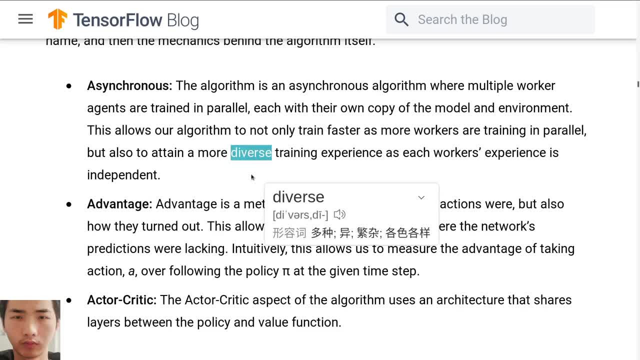 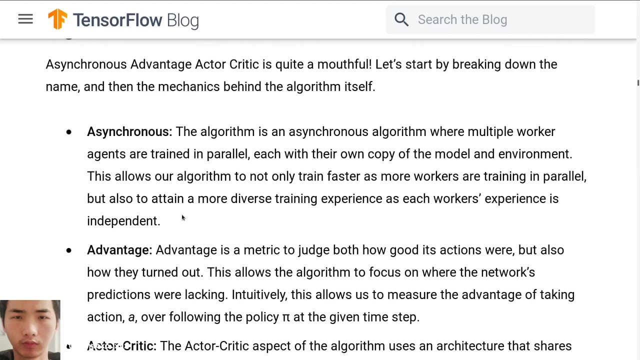 but also to attain a more diverse training experience, as each worker's experience is independent. Oh, now I know what the isynchro's advantage is. It's a multi-agent algorithm, I guess, And from this point I could know that in order to use 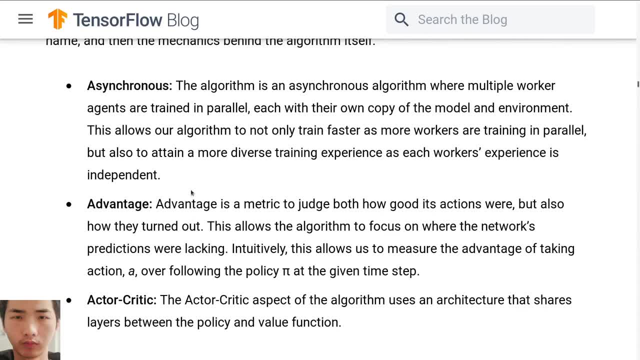 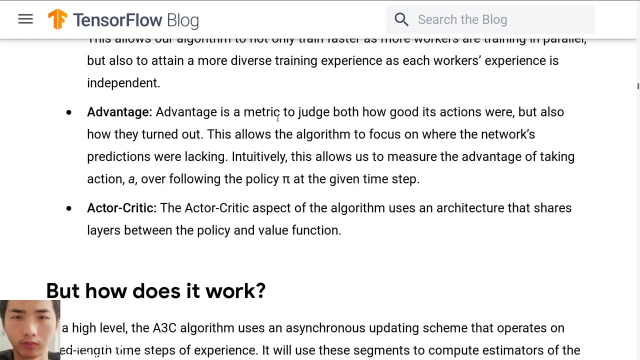 this algorithm you must have a strong GPU devices or computing devices, otherwise it won't work, because it got a beautiful agents. Isynchro's advantage is a metric to judge both how good its actions were, but also how they turned out. This allows the algorithm to focus on where the network's 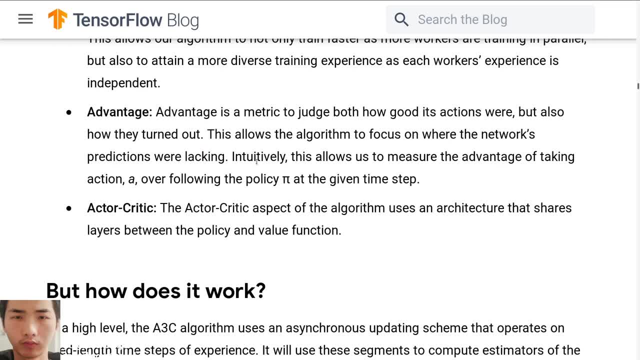 predictions were lacking Intuitively. this allows us to measure the advantage of taking action over following policy pie at the given time to reduce the risk of a better performance. This is what JSON is all about. It's an algorithm that can be used to get better results. 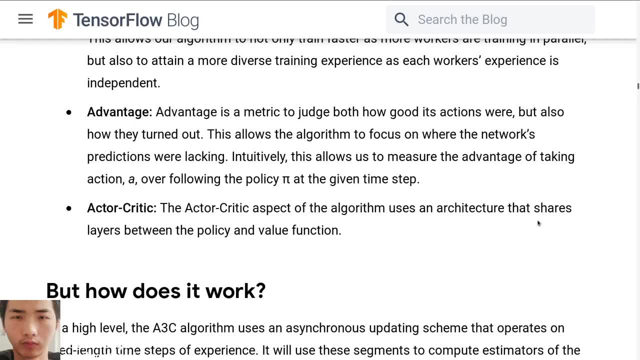 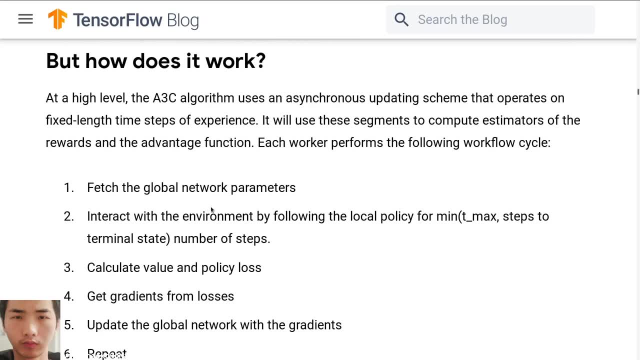 and have long-term results over time. On the other hand, the reason we didn't use the algorithm to tell us what was the Final Design of a certain property is also because the A3C algorithm is not developing a modern algorithm that is more advanced. 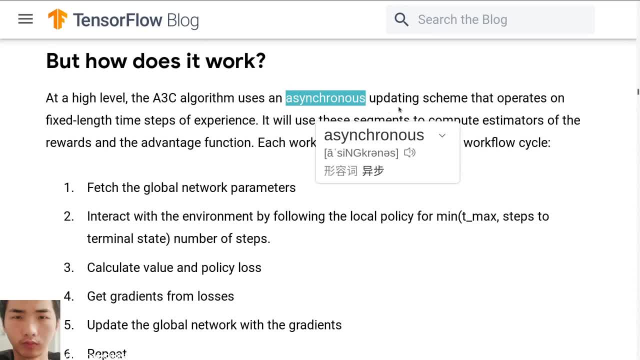 It's very easy to understand Because it has a very sophisticated ecosystem. as an updating scheme that operates on fixed-length 10 steps of experience, It will use these segments to compute estimators of the rewards and the advantage function. Each worker performs the following workflow cycle: 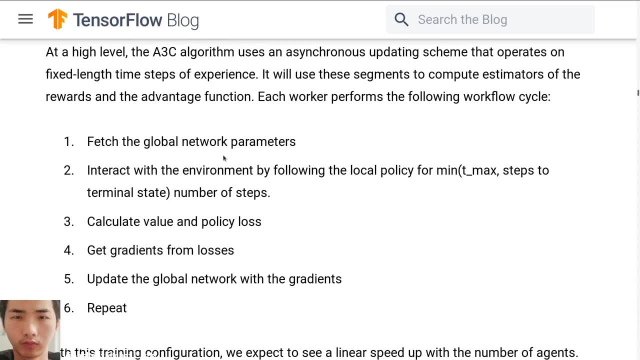 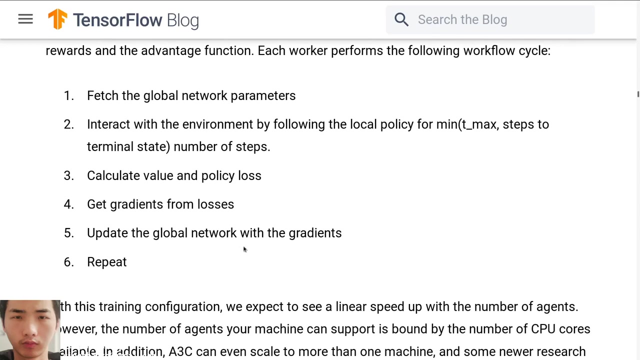 1. Fetch the global network parameters. 2. Interact with the environment by following local policy for number of steps, Tmax steps to terminal state. Calculate value and policy loss. Get gradients from losses. Update the global network with gradients. Repeat this process. 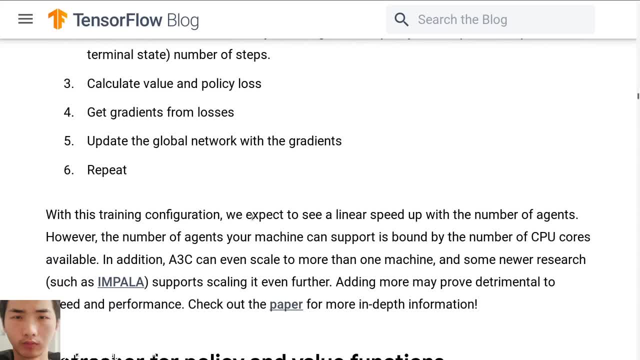 With this training configuration, we expect to see a linear speedup with the number of agents. However, the number of agents your machine can support is bound by the number of CPU cores available. Oh, in that case for my computer, my computer gets 4 CPU cores. 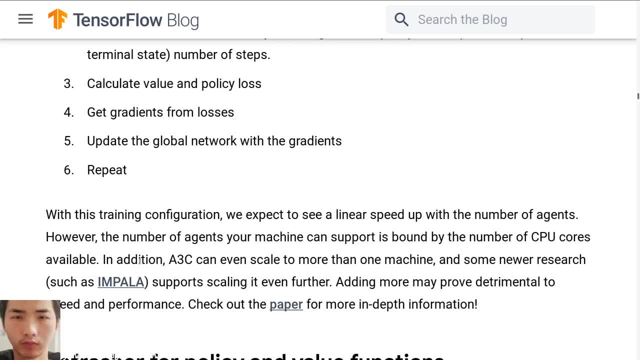 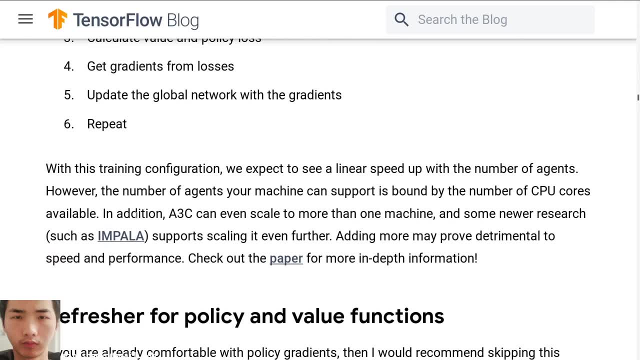 So to the maximum I could only use 4 agents if I want to use this algorithm. In addition, A3C can even scale to more than one machine And some newer research supports scaling it even further. Adding more may prove terminator to speed and performance. 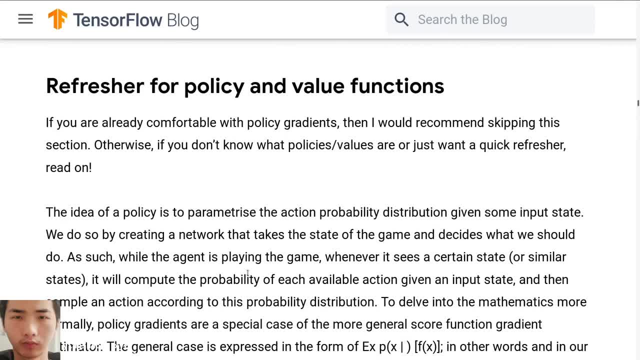 Great Refresher for policy and value functions. If you are already comfortable with policy gradients, then I would recommend skipping this section. Otherwise, if you don't know what policies or values are or just want a quick refresher, read on. 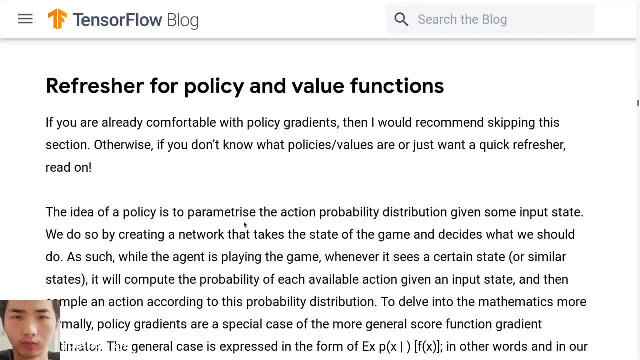 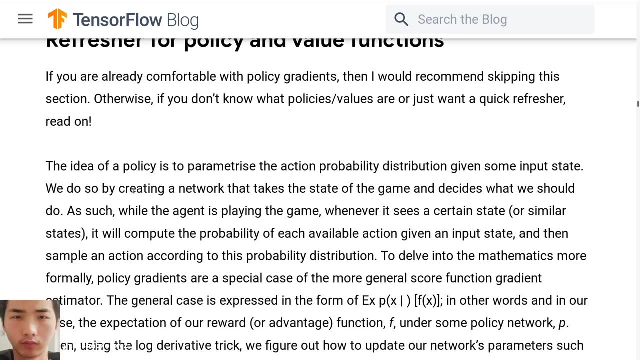 The idea of a policy is to parametrize the action probability distribution given some input states. We do so by creating a network that takes the state of the game and decides what we should do As such, while the agent is playing the game whenever it says a certain state or seminal state. 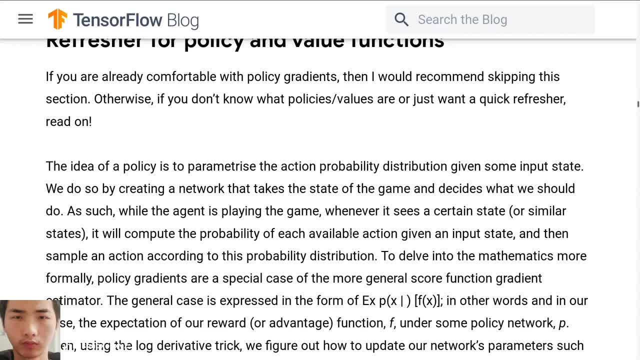 it will compute the probability of each available action given an input state and then sample an action according to this probability distribution. To delve into the mathematics more formally: policy gradients are a special case of a game. Policy gradients are a special case of a game. 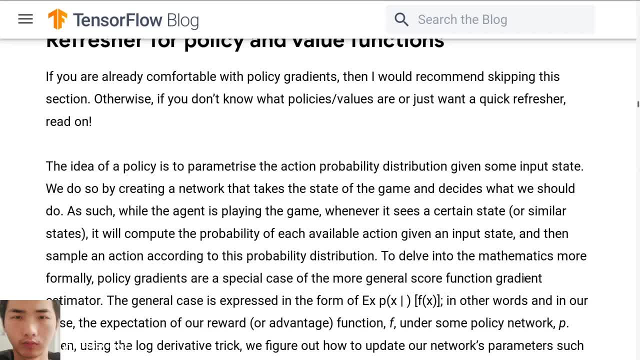 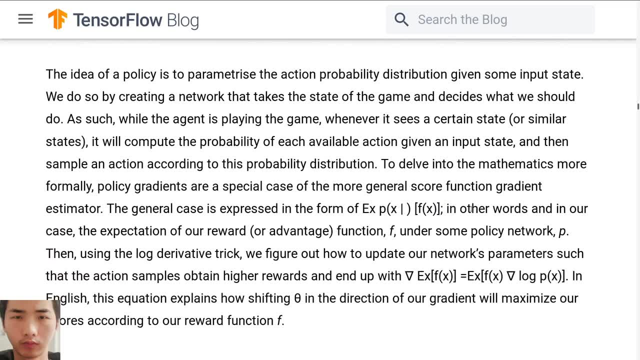 The most common case of a game is the general score function of the more general score function, gradient estimator. The general case is expressed in the form of this, In other words, and in our case, the expectation of a reward function f under some policy network, P. 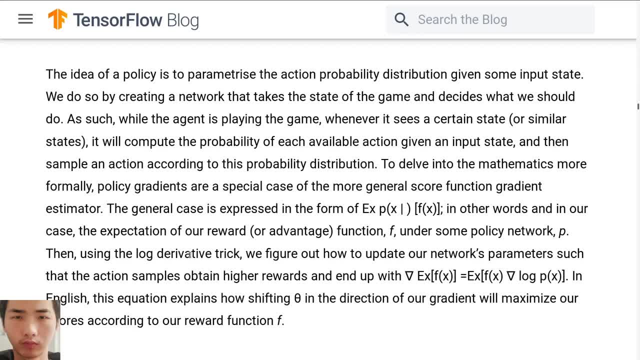 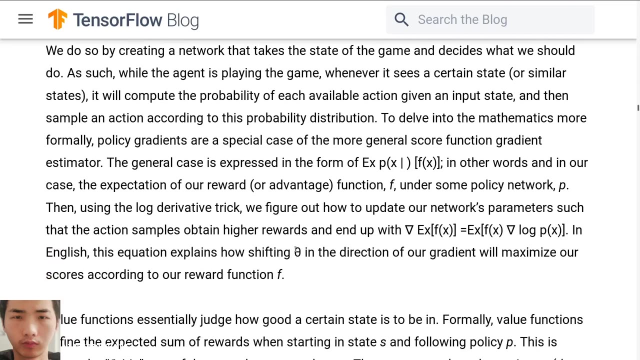 Then, using the log derivative tree, we figure out how to update our network, update our network's parameters such that the action samples obtain higher rewards, and end up with an expression like this In English: this equation explains how shifting beta in the direction of our gradient will. 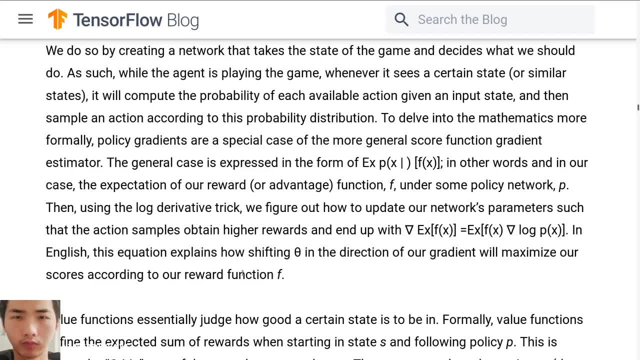 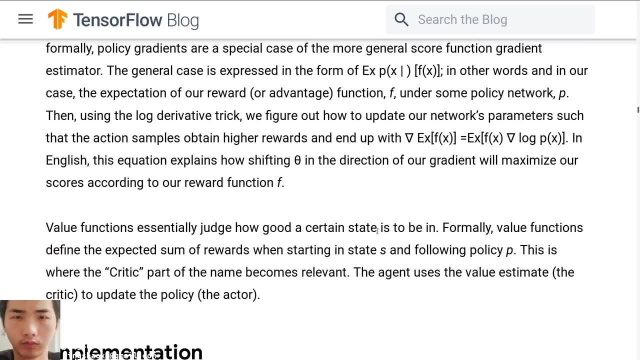 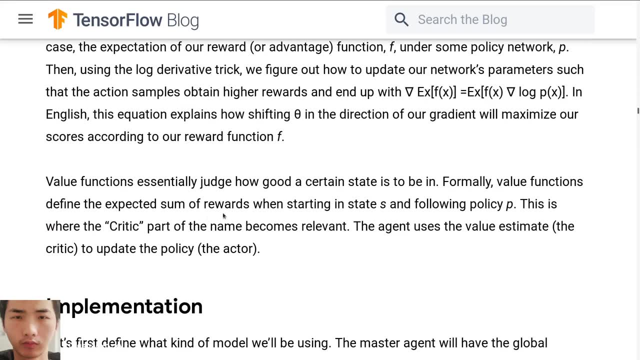 maximize our scores according to the reward function. f. Value functions essentially judge how good a certain state is to be. Formally, value functions define the expected sum of rewards when starting in state s and following policy p. This is where the critic part of the lem becomes relevant. The 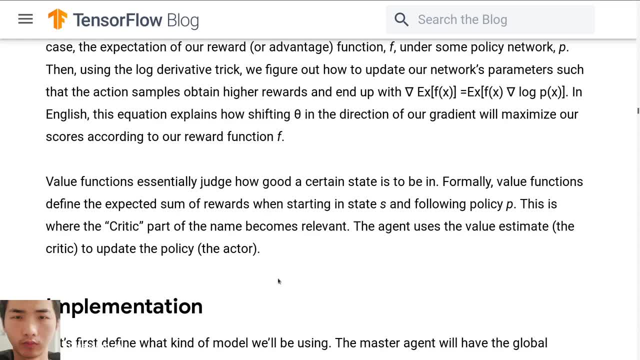 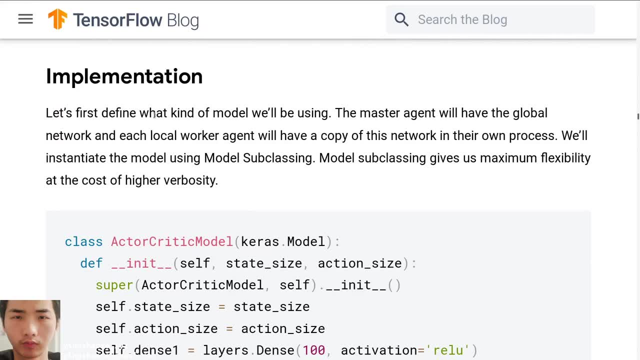 agent uses the value estimate to update the policy. Let's talk about the implementation, of methods For implementation. let's first define what kind of model we'll be using. The master agent will have the global network and each local worker agent will have a copy of this network. 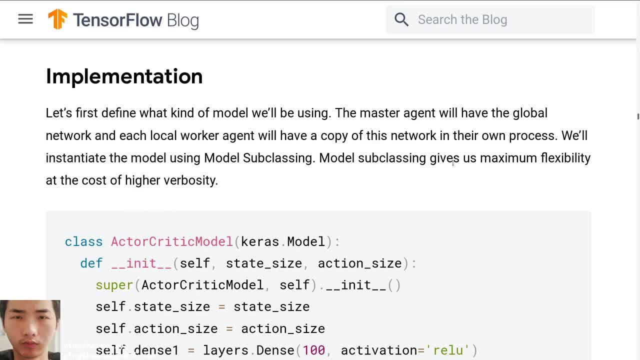 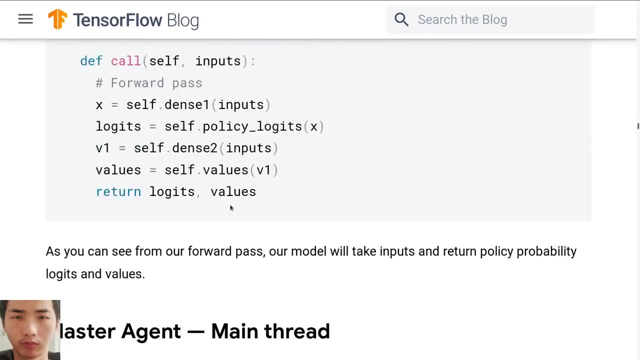 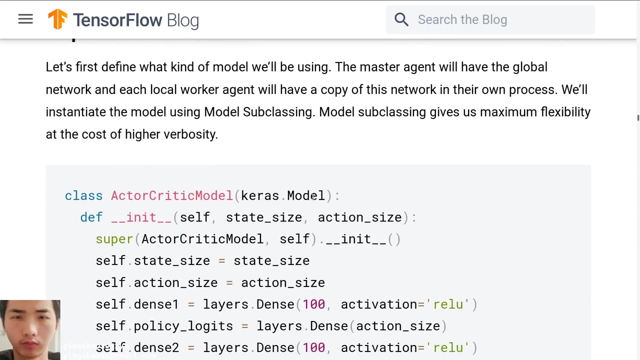 in their own process. We will Inefficiently use the model using model subclassing. A model subclassing gives us the following: maximum flexibility to at the cost of a higher verbosity. great, here we can have a simple glass at the, the carousel model of function. I mean how to use it with. 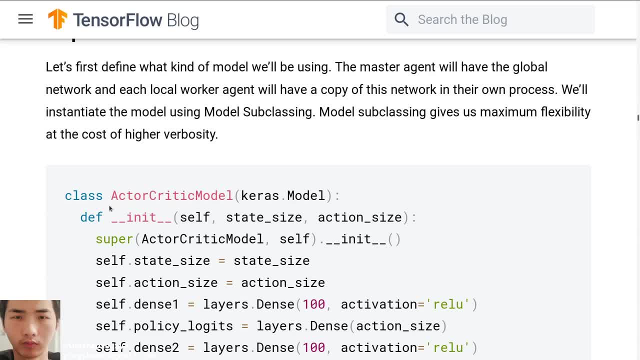 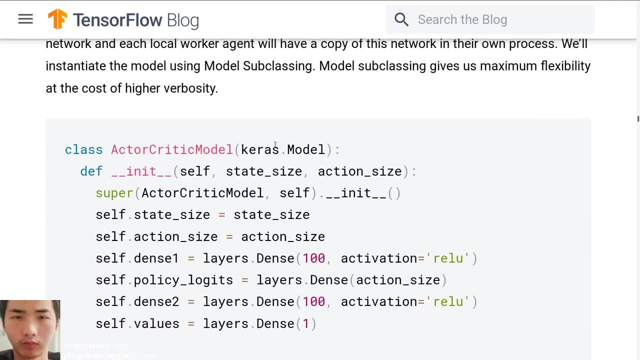 with with the, the subclass stuff here. the initial function is it will take two, two parameters: the state size, the action size. super actor created a critic model in natural. yeah, that means we have to initiate the carousel model and predefined the initial function first. then we give the two parameters state. 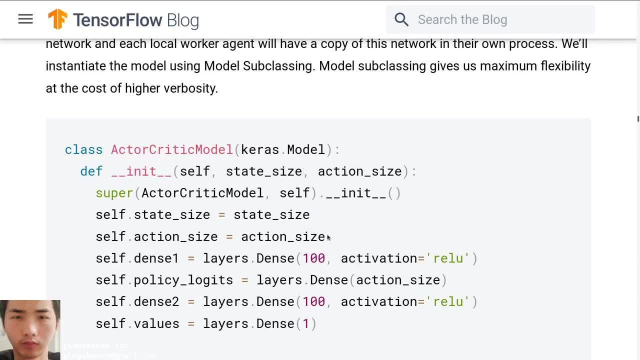 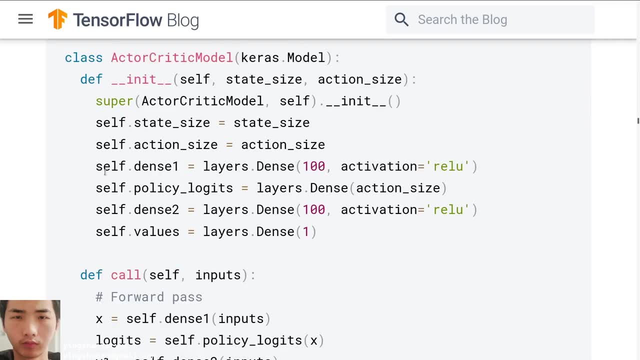 size and the action size to to the class, so we can use it later in the class function. self that dance, one equal to layers. that dance with one hundred hundred, with the size of 100, the activation function, equal to our eli you. so that's the first player, I guess, or maybe it's not, because we are doing eight with. 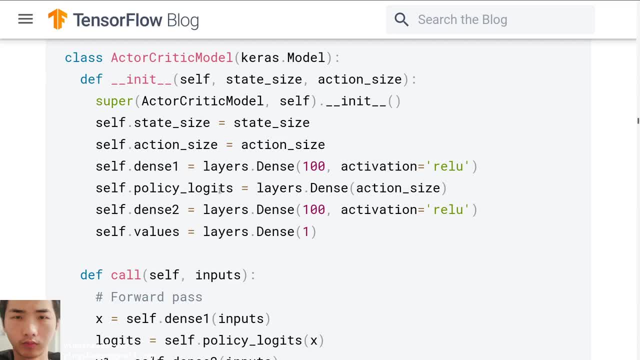 technology, subcussing technology. then we define the policy lei, equal to the layers to dance with action, their using values, delivery, Send in bounds to the class to KNOW what gods. But as soon as class technology we can agree with, this doesn't need to be a. 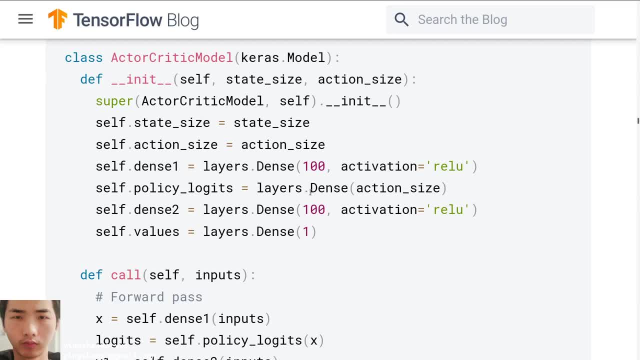 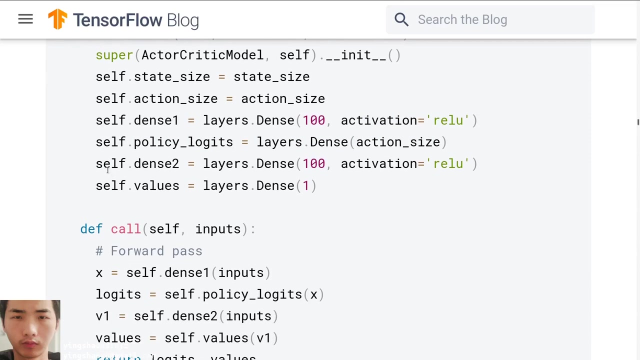 size So it may somehow output you the action, how many actions you have, For how many actions we have. this layer will output that many or full actions. Then we define: the dense2 layer is also a 100 size of dense layer with the activation. 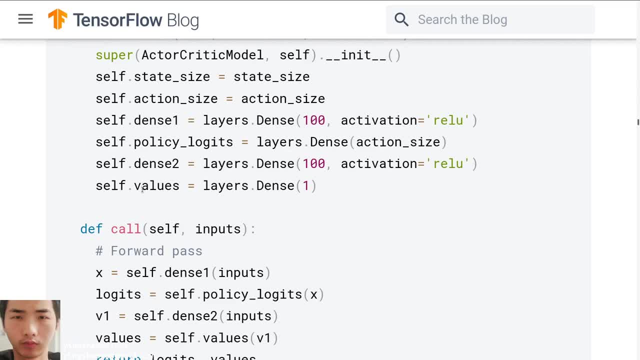 function of relu And the values. well, the values, let's say, it represents. for by giving, no matter what kind of states you give it, to this model, it will, you know, return your value, And that value represents the reward, How many rewards you can get by doing. 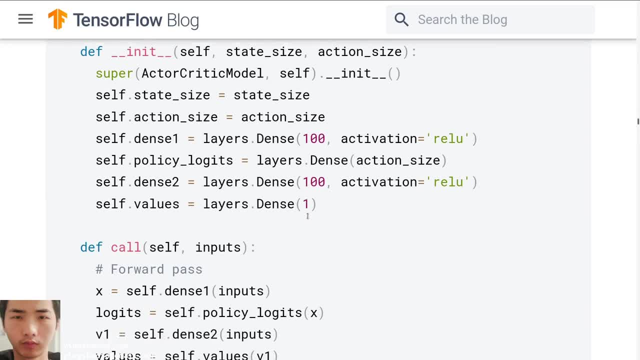 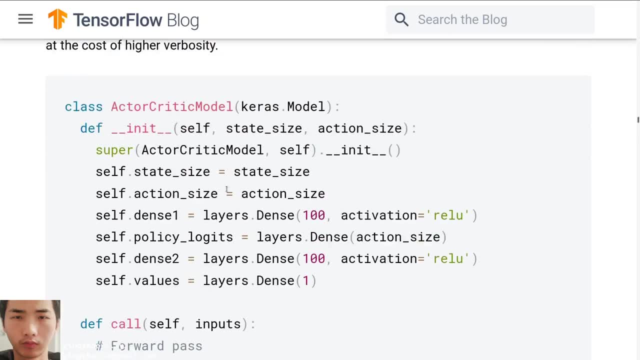 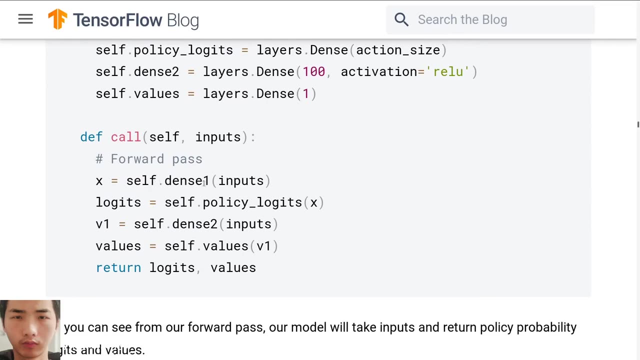 that action or kind of things like that. And then another function call function. for this function it will take the inputs as a parameter. Then x equal to selfdense1, it takes the inputs as the inputs. it will output X, and for X we will add another layer. it's a. 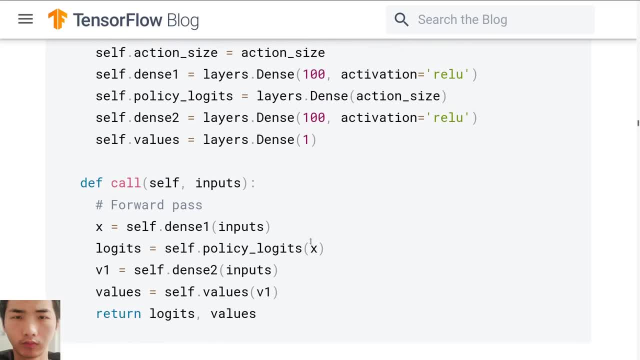 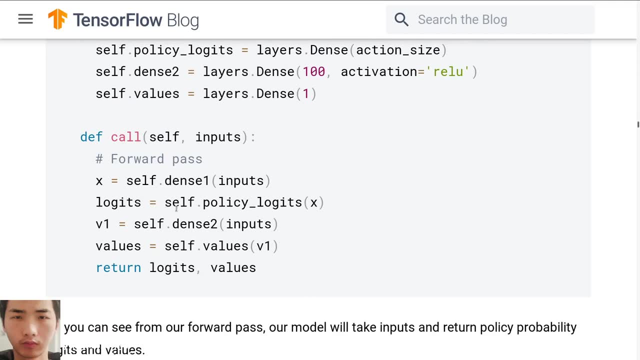 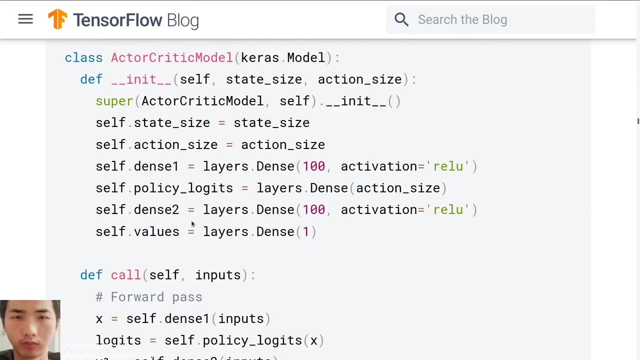 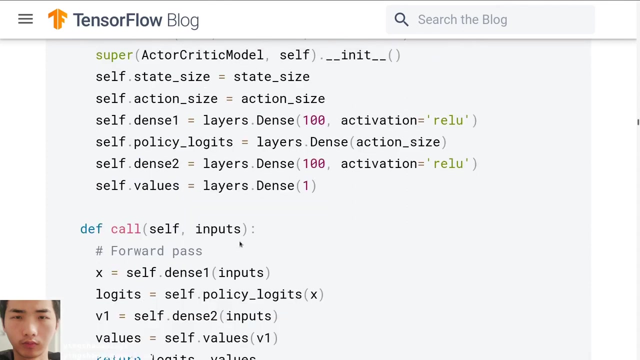 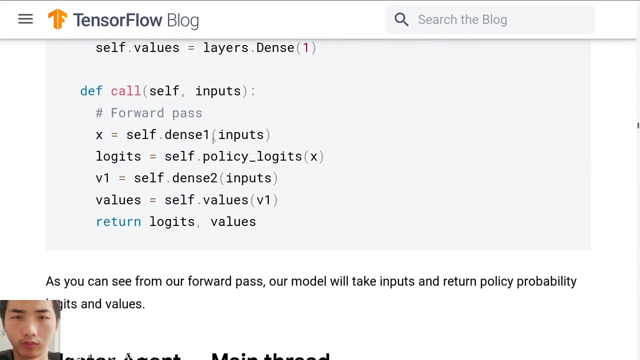 policy logits layer and for this layer it will output the logics it is outputs. so, as now, as I say, this is just like the functional API in Keras. it is the same, especially under the core function. first you define your layers at the initiate function, then you do the the chain operation, I mean you. 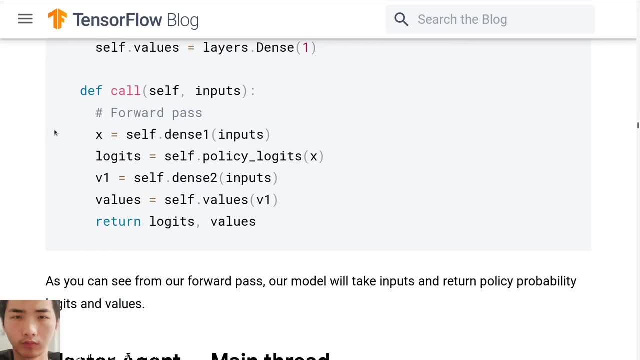 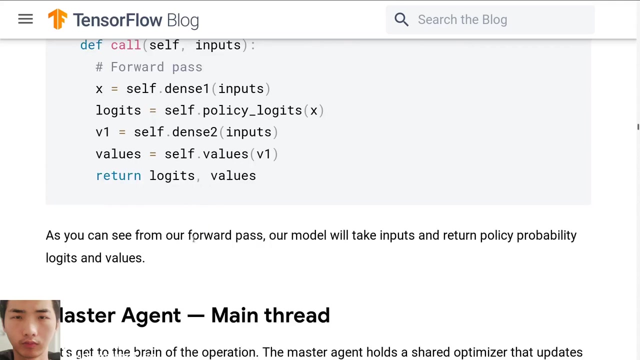 take the inputs, you get the outputs then then the first layers outputs will be used as the second layers inputs- right, it's all the same. and finally, you return the logits, which is the actions. then you return the values. as you can see, from our forward path, our model will: 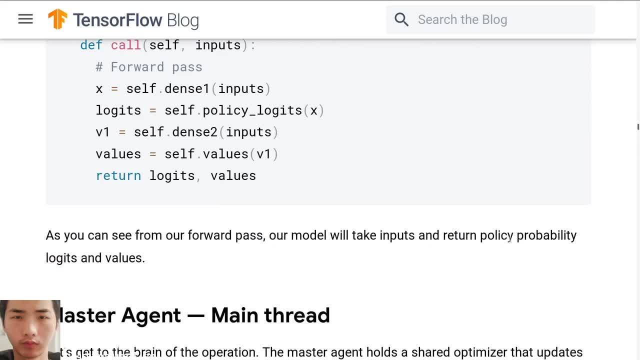 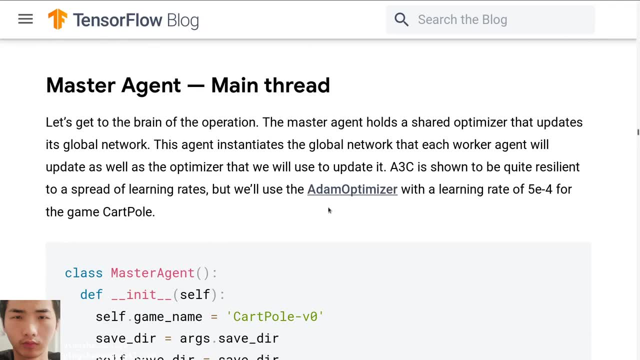 take inputs and return policy, probability logits and values. master agent- main street. let's get to the brain of the operation. the master agent holds a shared optimizer that updates its global network. this agent instantiator acts the global network that each Walker agent will update, as well as the optimizer that we 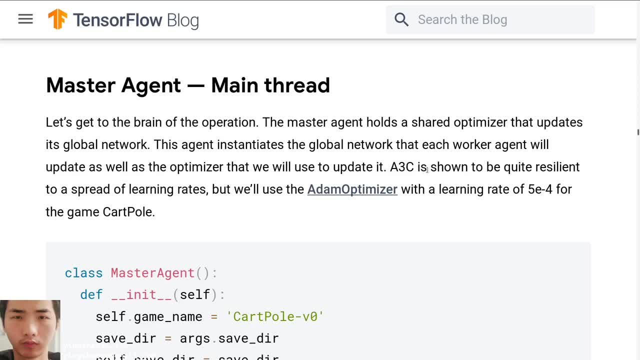 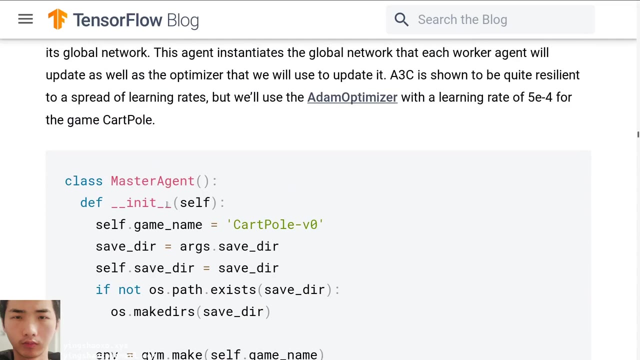 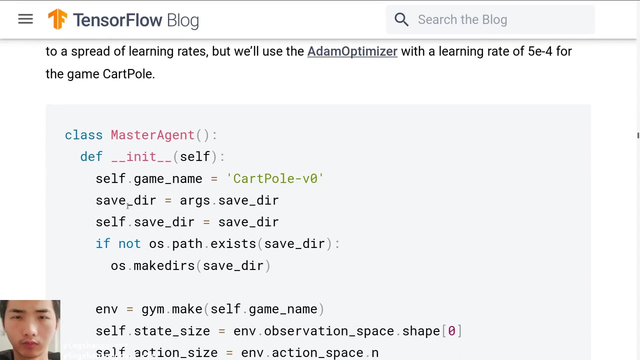 were used to update aids. else, say, is shown to be quite resilient to a spirit of learning rate, But I will use the ADAM optimizer with a learning rate of this for the game. The master agent is a class. For this class, the gameName equal to carPerl. The save directory. 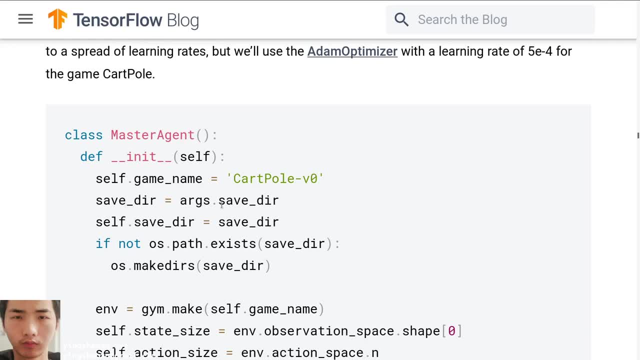 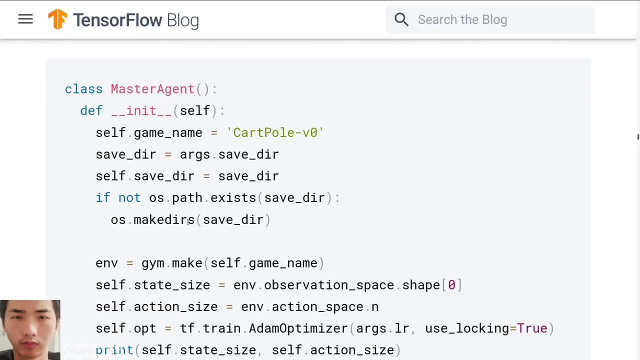 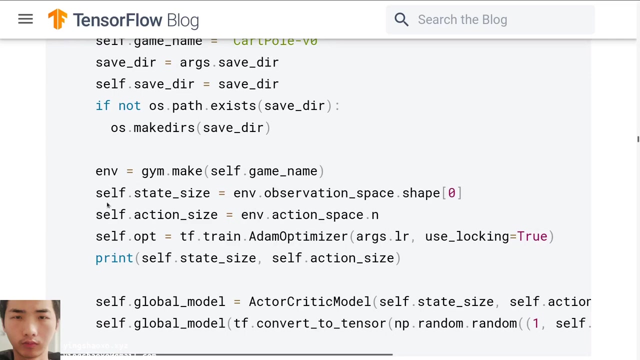 equal to a directory. pass The save that. no Yeah, If that pass was not existed, we would say we want to make a new directory. Then we create the environment based on the gameName. We say the state size equal to the environment. 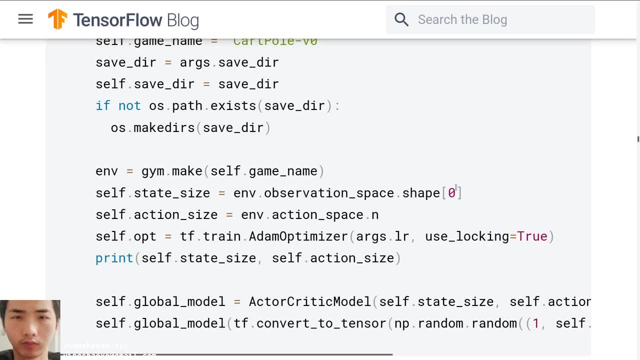 that observationSpec. So we create the environment based on the gameName. We say the state size equal to the environment that observationSpec. So we create the environment based on the gameName. We say the state size equal to the environment that observationSpacen. 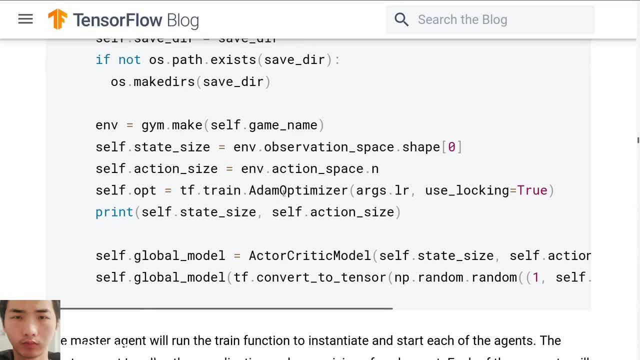 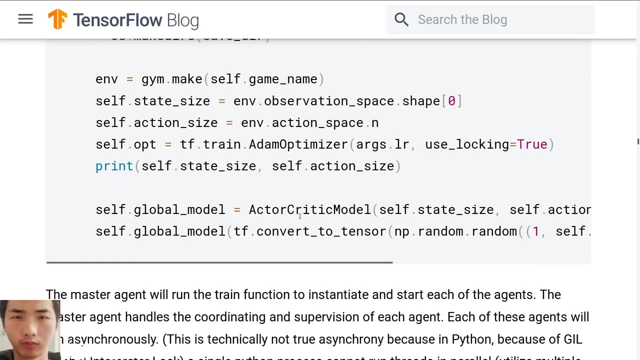 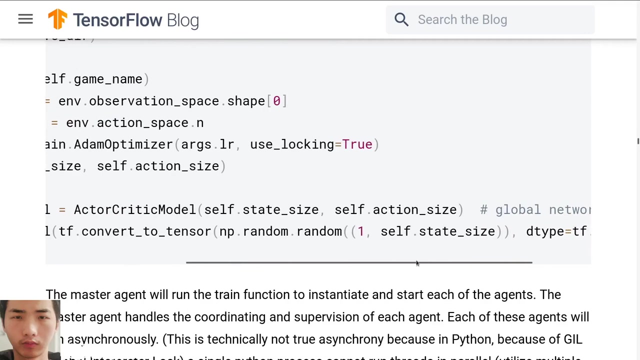 The optimizer equal to tftrainadminoptimizer. The learning rate useLogin- equal to true. We print out the state size and action size. The global model, equal to the actor created model, by giving it the state size and action size. Then we instantiate the. 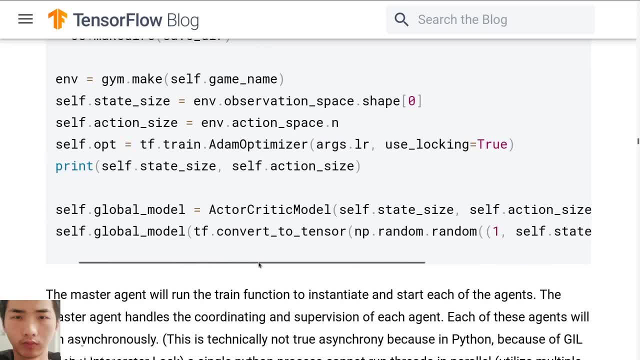 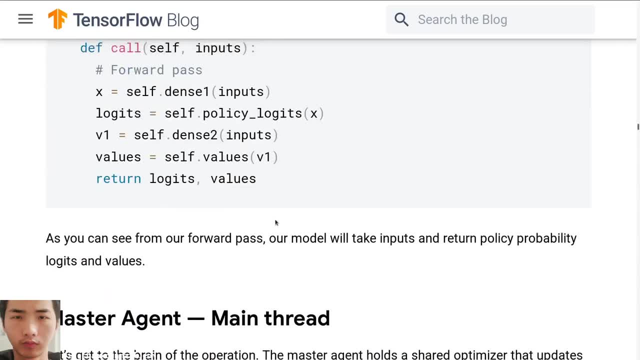 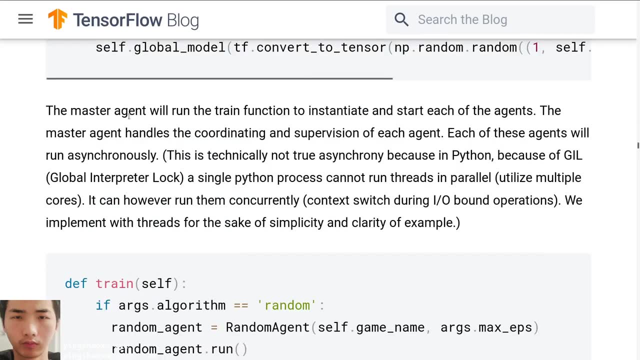 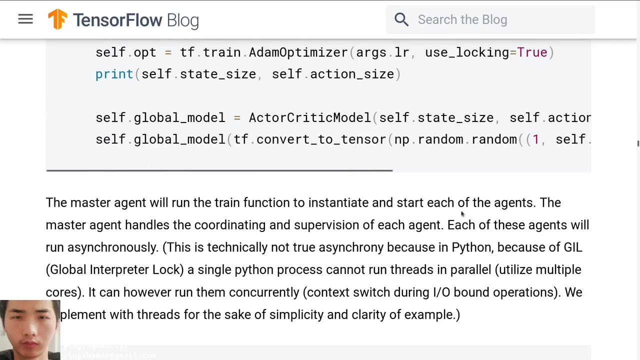 model by giving it the proper parameters. So for this class ActorCriticModel we actually define it at the borrow. The master agent will run the train function to instantiate and start each of the agents. The master agent handles the according and separation of each agent. Each of these agents will run. 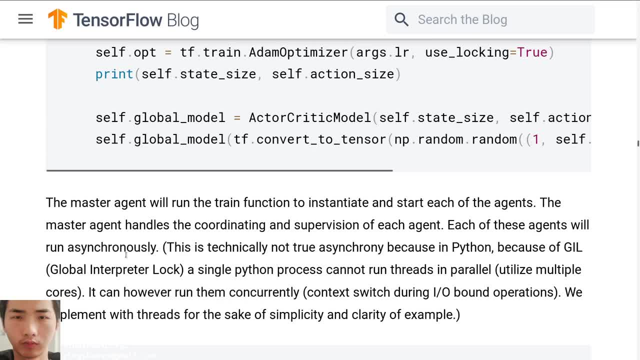 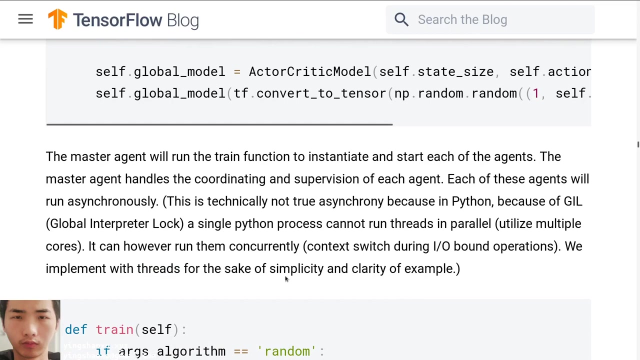 asynchronously. This is technically not true asynchrony because in Python, because of the GIO globe interpreter lock, a single Python process cannot run threads in parallel. It can, however, run the concurrently context switch during IO bound operations with implements with threads. and for the sake of simplicity and clarity of example, 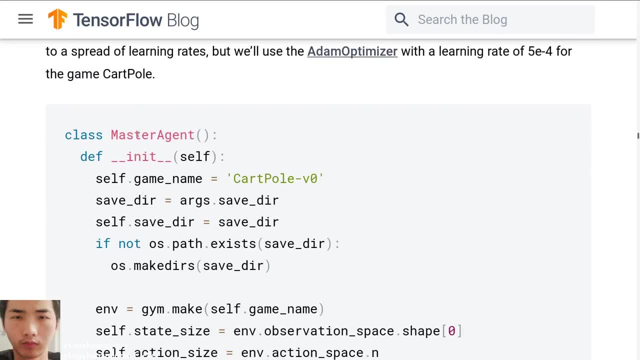 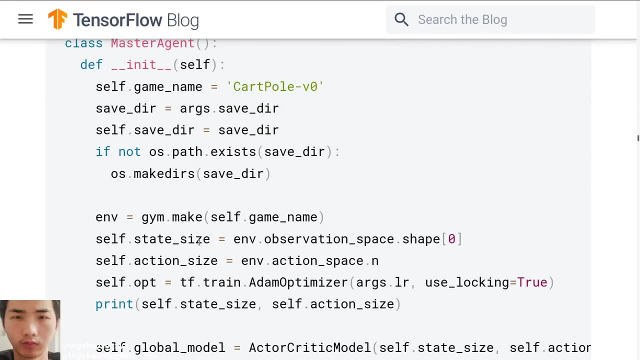 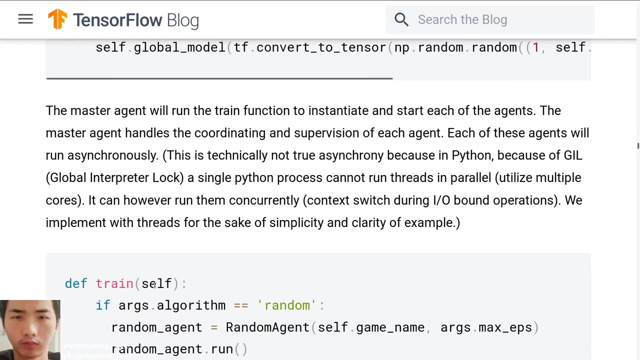 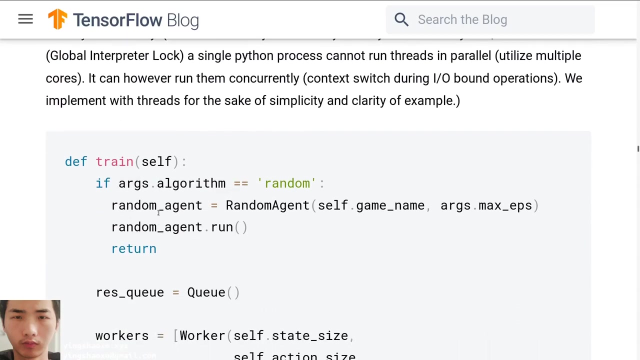 So this is the same class. We are in the master agent. We haven't done yet. This is the initial process. We define the global model and we instantiate the global model. Then we have to define functions for that class. So here is a function, hang функ. If the arguments that 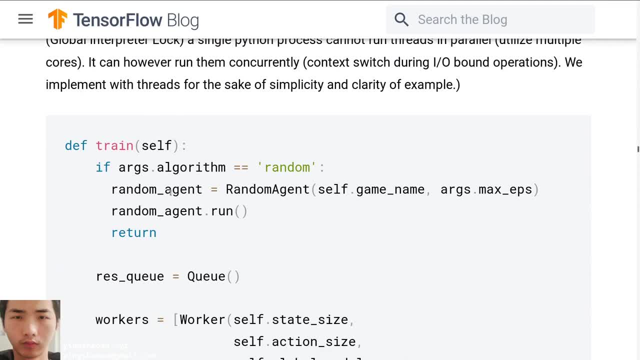 accuracy equal to readr. then we say: readr agent, equal to readr agent. with the, the, the environment, lvl and maxed episodes, we run that agent, That, that readr agent. After that we return: itrzeatoqzeatoqzeatoq. 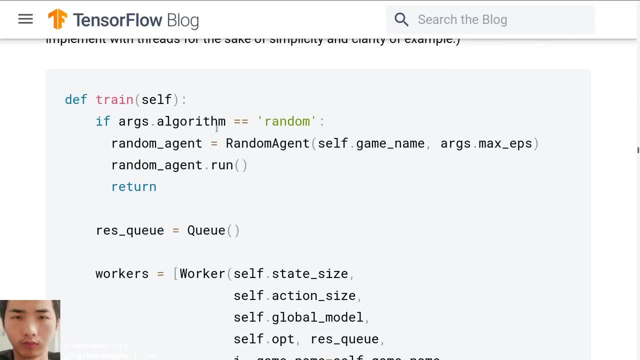 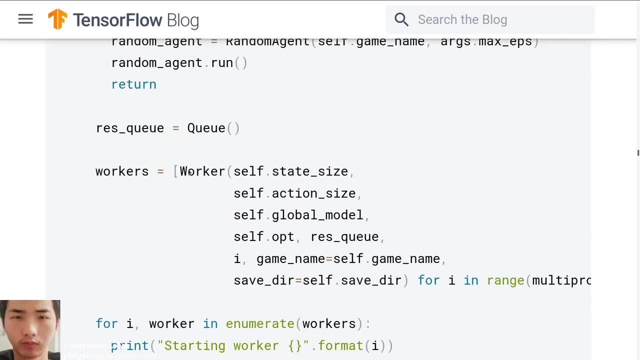 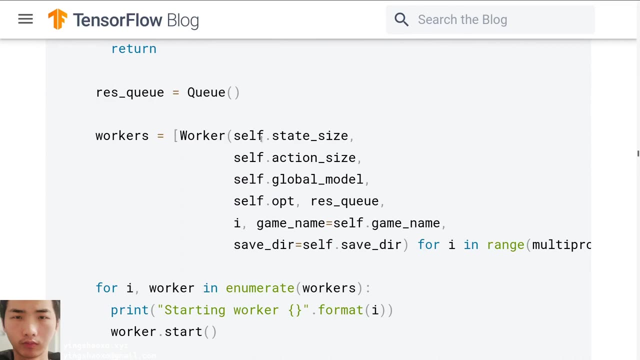 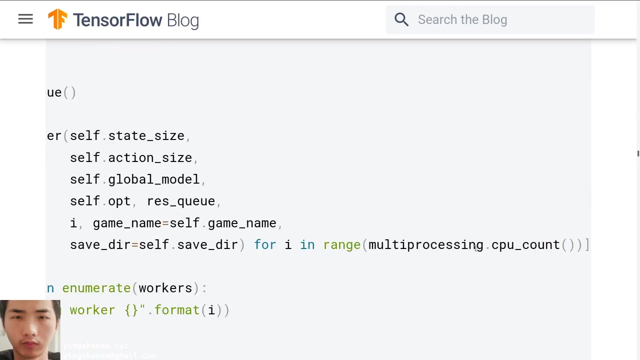 Ann�, cel not equal to written. we'll say the queue equal to a new queue data structure. a pipeline Workers equal to worker of a lot of things. It all depends on how many CPU cores we have. We use this function to get our CPU cores. Yeah, but here's the problem. I don't know. 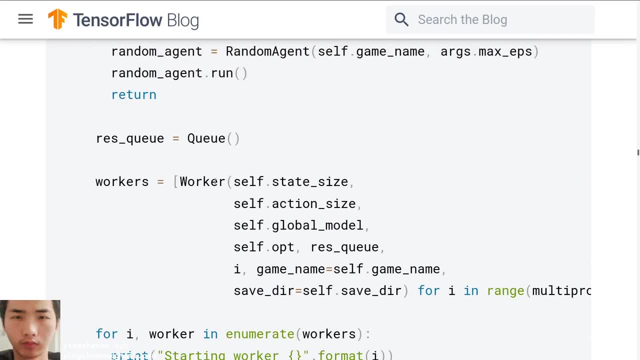 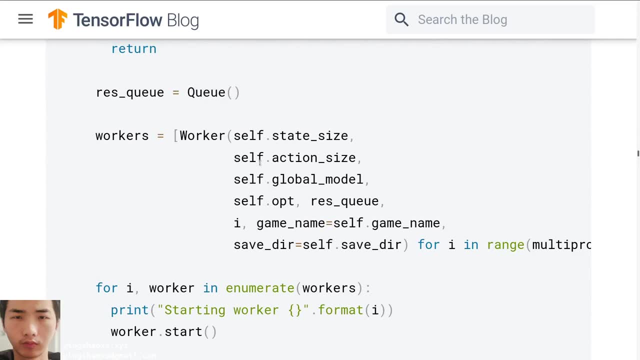 where the worker class or function comes from. We haven't defined it right, But doesn't matter. Let's say it takes the state size, the action size, the global model, and optimizes the queue data structure and the environment length, the 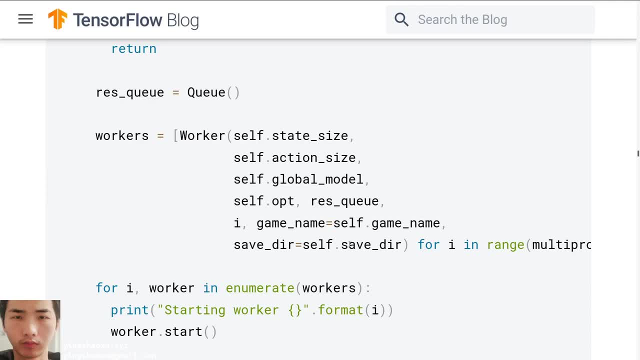 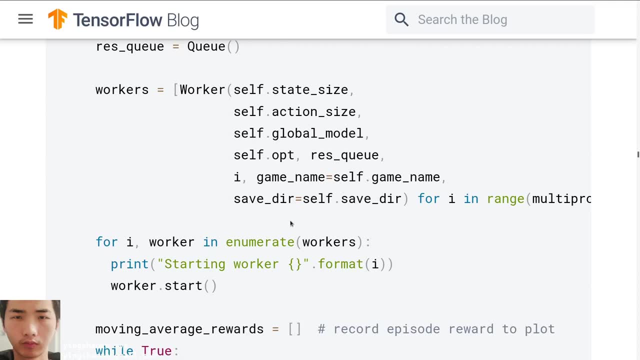 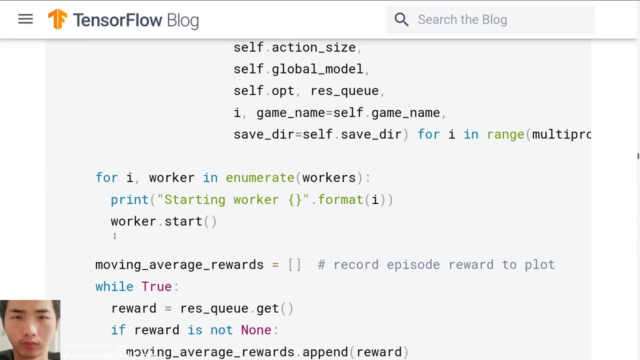 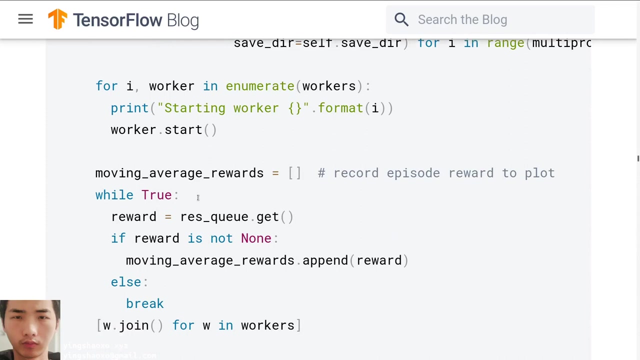 saved data structure, You know, for each worker it may have a different dictionary for saving its data. For I worker, you know, for worker, in workers we start each worker Moving average rewards equal to an empty. last. We'll choose- we do a loop here- The reward equal to the. 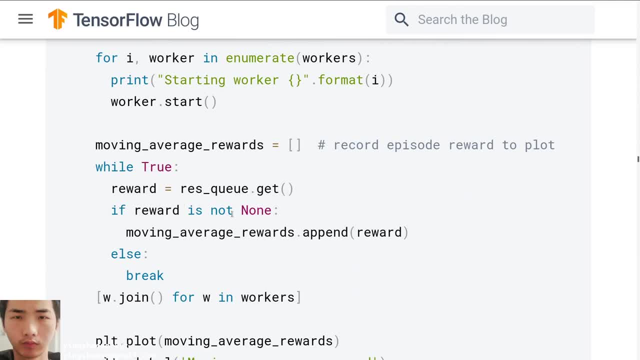 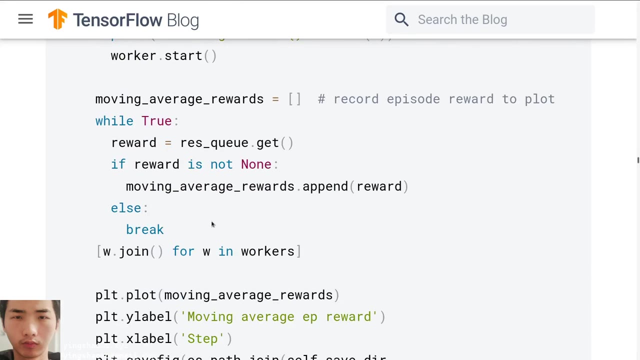 queue data structure That gets if reward is not known. if it's not known, we add that reward to the average rewards last And in the end I guess we have to calculate the average rewards later. Yeah, if the reward is known, we break that. Then we join all those. 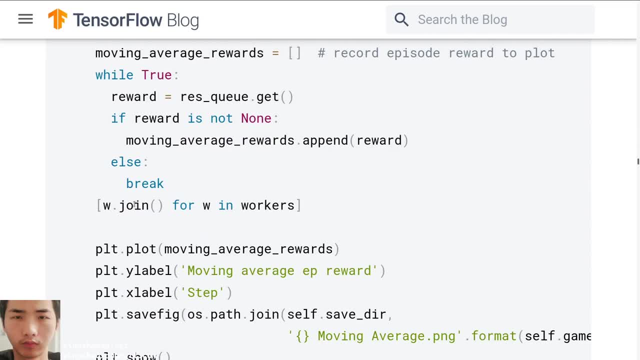 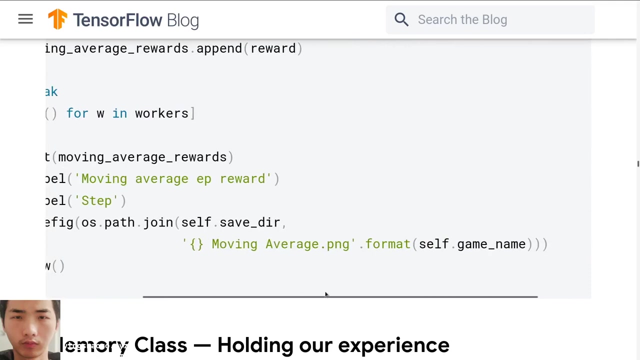 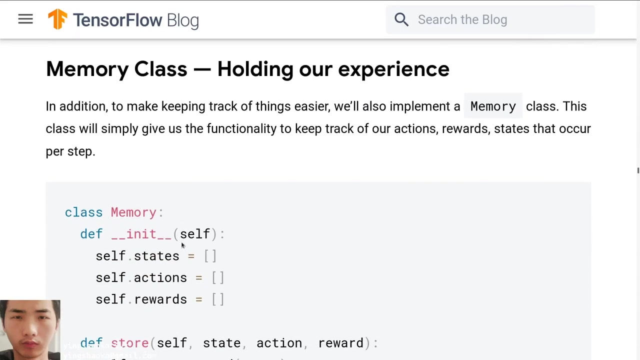 I don't know if it's a multi-process or something like that, But we will join those process into this main process by using this line of code. Then we do a graph drawing, We draw out the words, I don't know. So we can see at this point that we want to show here at each one of the 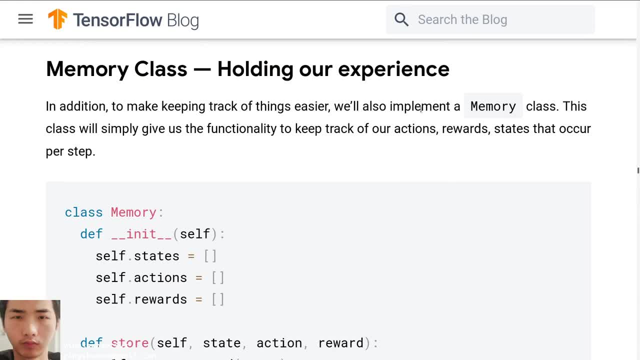 rows. we are pretty happy with the results. And if we finish it, what can we say? Forget about theinnumerableissy. Read out the sounds in A to B: equals day, Okay, OK. So here is the separated вет senhor, dancing later with you. Maybe it's a little Taylor House, right. Maybe it's a little Hitler House, right. Wasn't your India? didn't you have an A? Yeah, there's Texas and I think I've got a challenge to this. But if you have any questioning between a model and a graph, like a probabilityオigne, 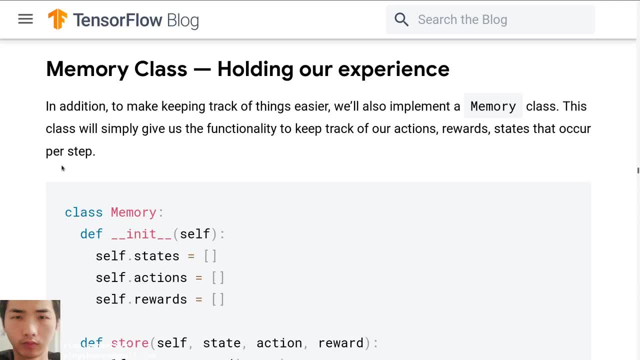 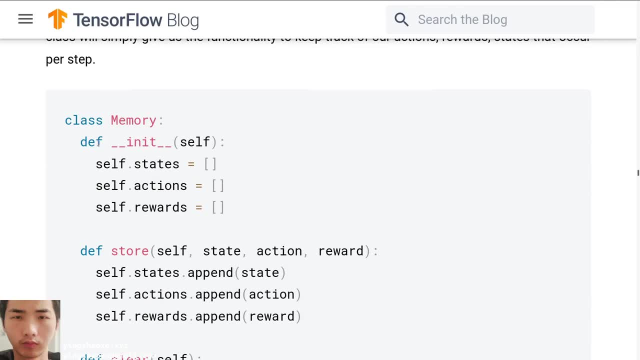 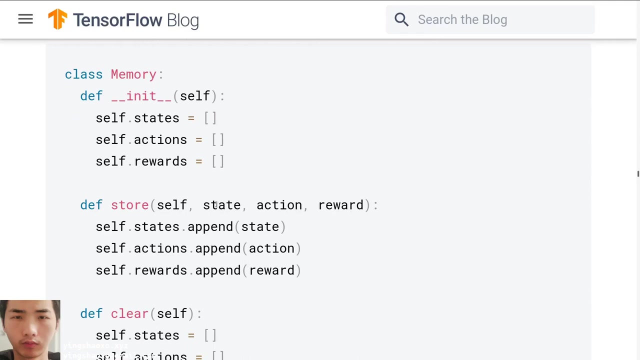 rewards and states that occur per step. Here's a class of of memory. First we define the initial function: states, actions, the rewards, it's all lasts. Define a store function: It is simple. we just have to add the state, the. 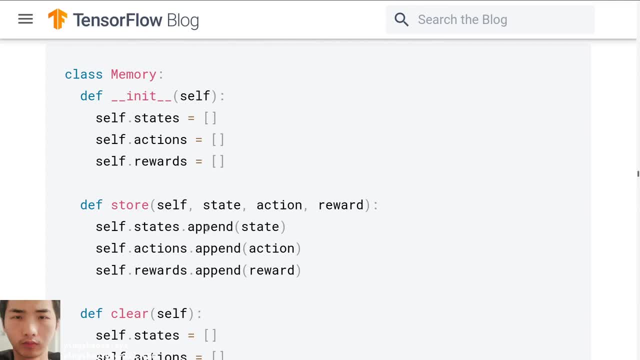 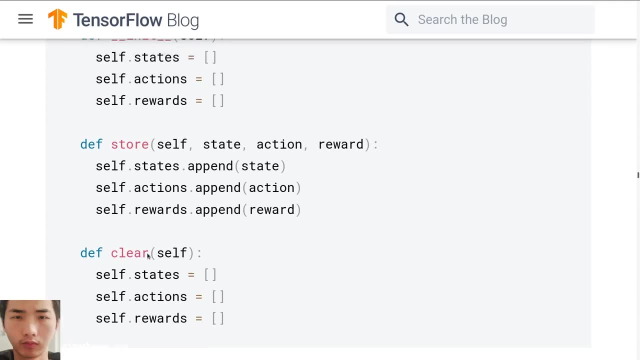 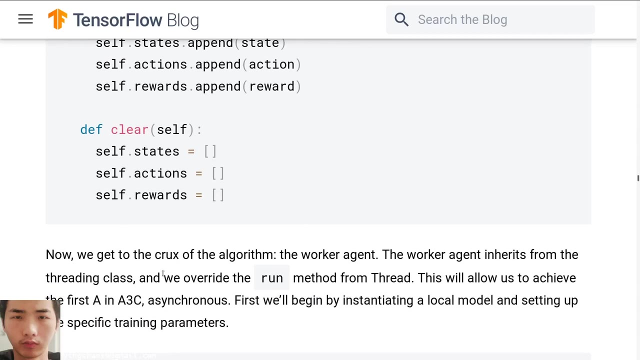 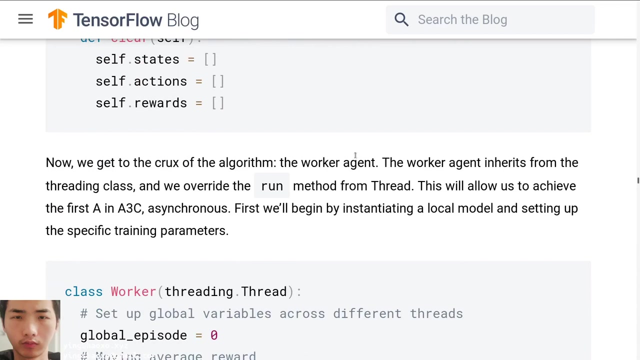 action, the reward to three lasts. Then we define the clear function. It is also very simple: we just have to empty the three lasts states action reward. Now we get to the critical part of the algorithm: the worker agent, The worker. 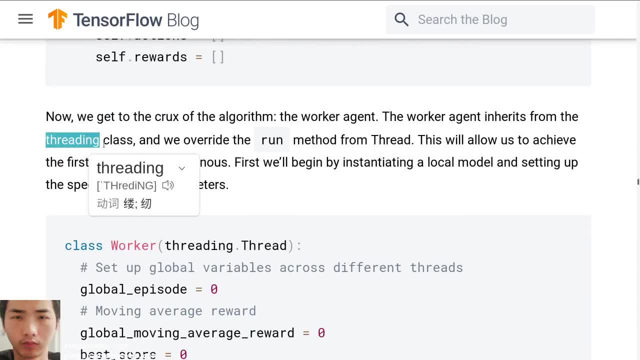 agent inherits from the strategy. We start creating a threading class and we override the wrong method from thread. This will allow us to achieve the first A in A3C: asynchronous. First we will begin by initializing a local model and setting up the specific training. 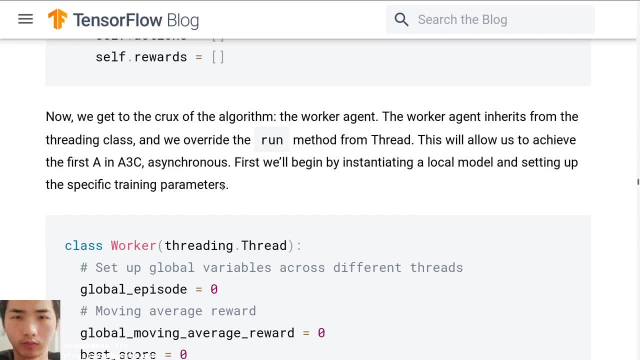 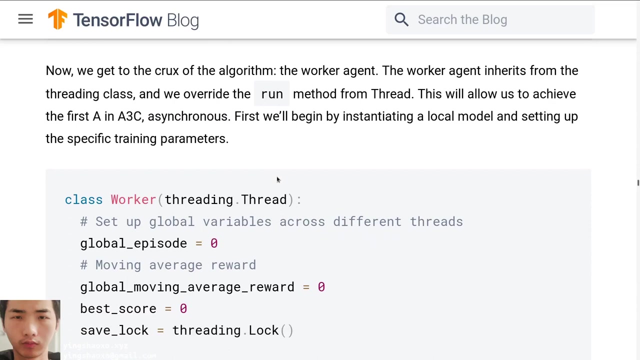 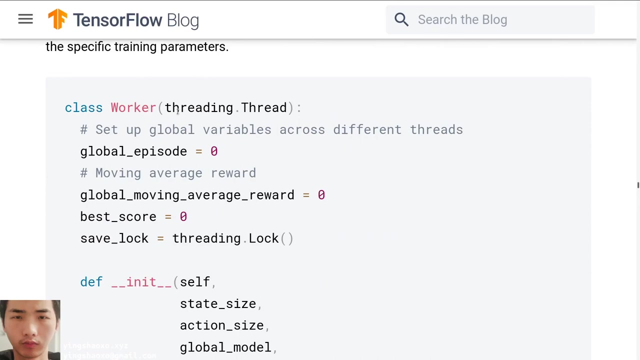 parameters. So now I understood that for this post they are using the threading techniques to achieve the asynchronous in this algorithm. They are not using multiprocessing, but the threading technique. Okay, now let's define the worker class. The worker class is inherited from the threadingthread. 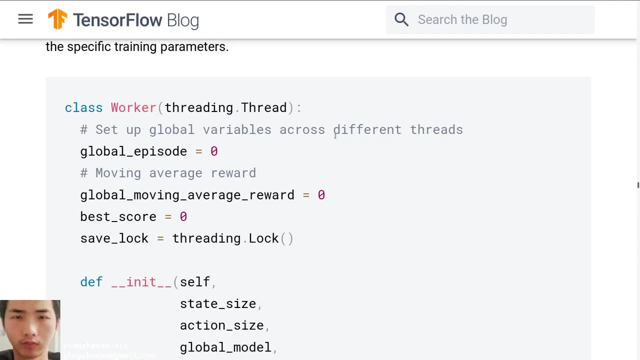 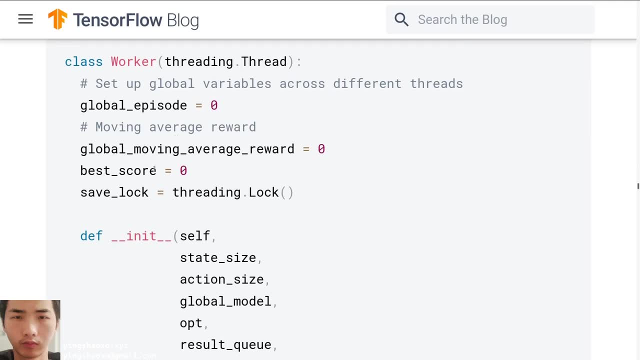 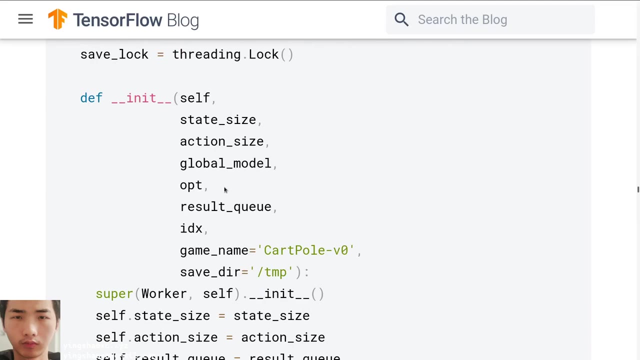 We have to set up the global variables across different sorts: The global episode equal to 0, the moving average reward equal to 0,. the best score equal to 0,. the save log equal to the threadinglog. We define the parameters that this worker need to receive. 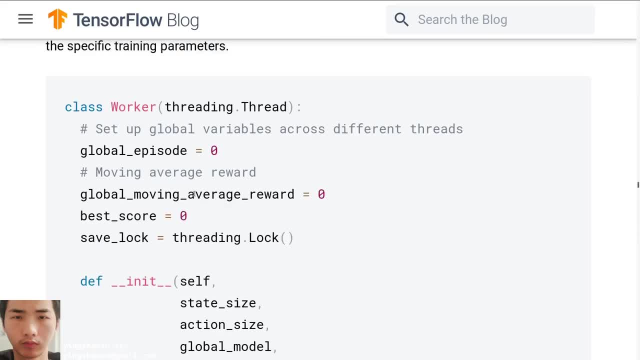 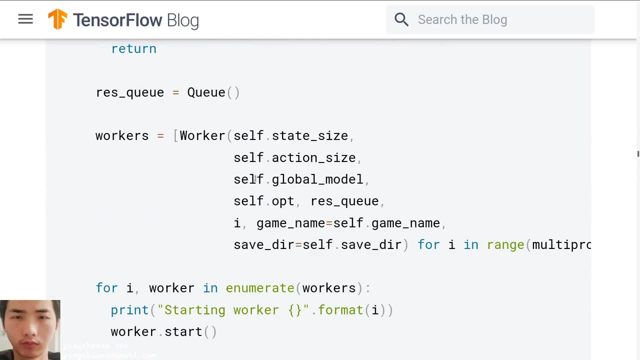 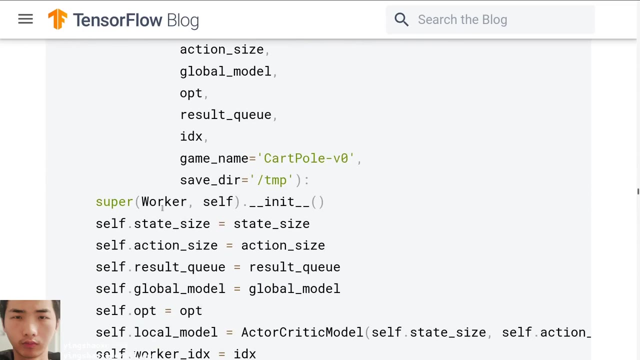 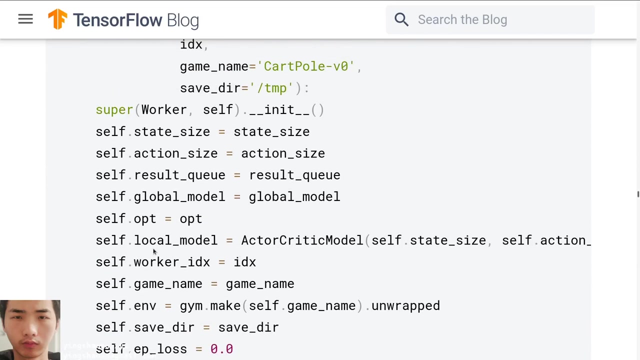 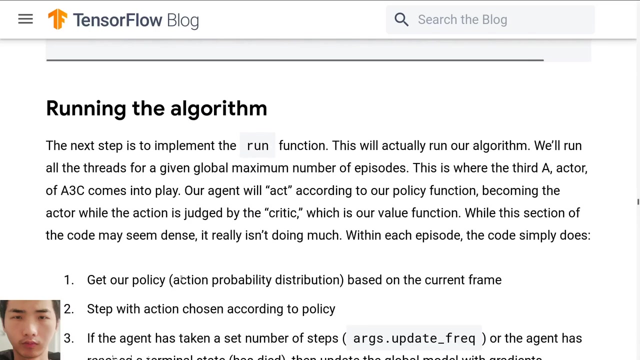 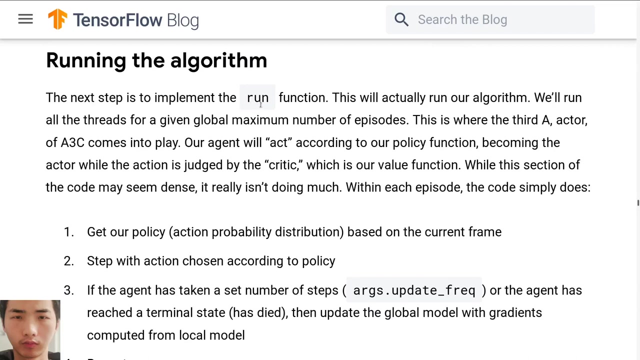 It is the same as we call it in here. It is the same. We have to give it that much of parameters. Okay, after we initiate the global superclass, We define our local model by using the actor critical model running the algorithm. The next step is to implement the run function. 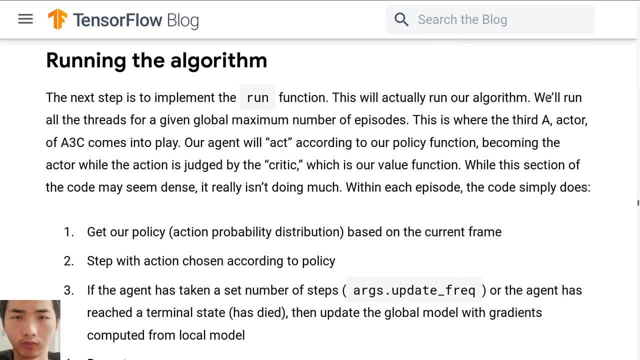 This will actually run. our algorithm Will run all the threads for a given global maximum number of episodes. This is where the third A actor of A3C comes into play. Our agent will act according to our policy function, becoming the actor while the action. 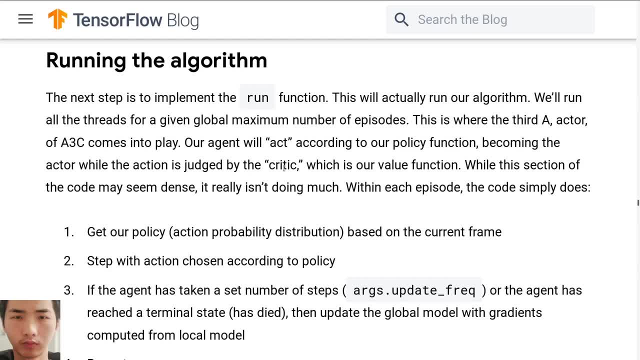 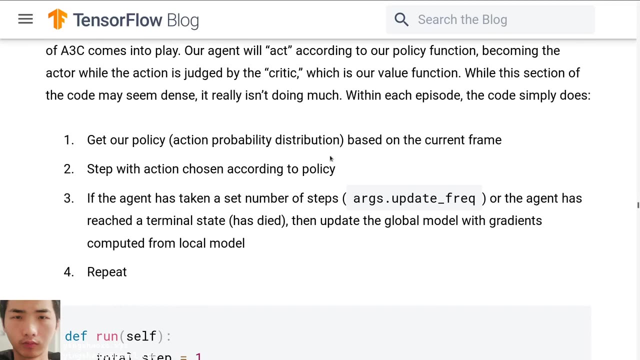 is judged by the critic, which is our value function. While this section of the code may seem dense, it really isn't doing much Within each episode. The code Basically does: 1. Get our policy, I mean the action probability distribution based on the current frame. 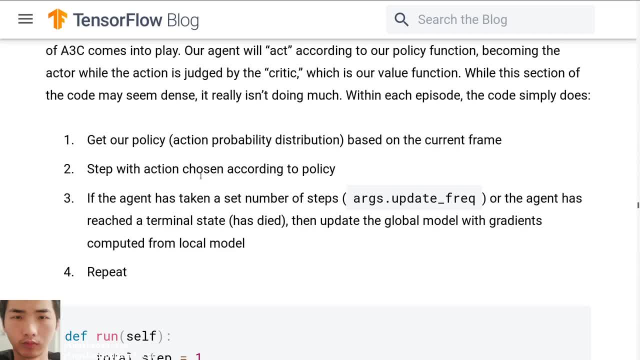 2. Steep with action chosen according to policy. 3. If the agent has taken a set number of steps, Or the agent has reached a terminal state, Has that Then update the global model with gradients computed from the local model. 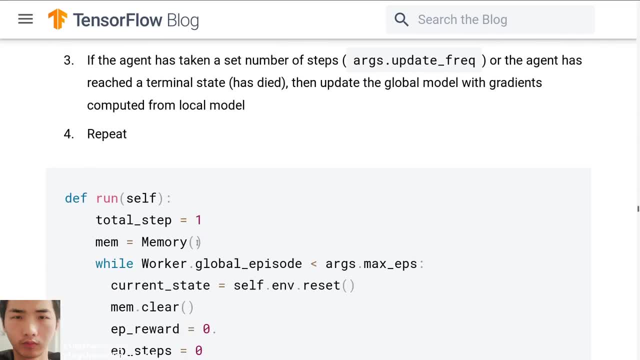 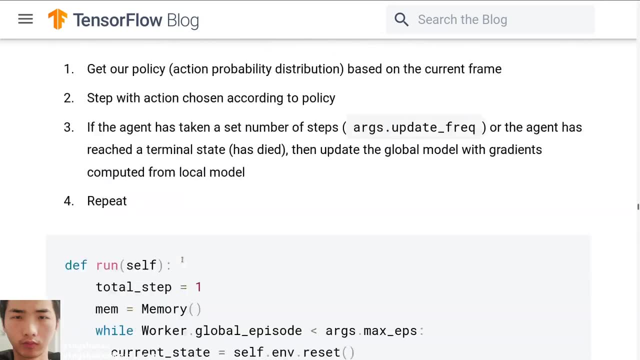 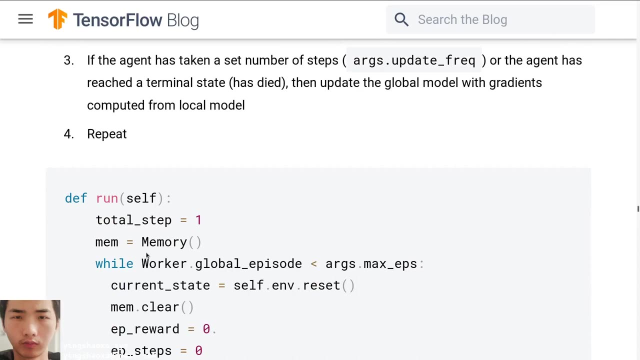 4. Repeat the whole process. So let's define our run function. It's quite long at the code side but we will conquer it. We will break it down into pieces and try to understand that The run function, The total step equal to 1.. 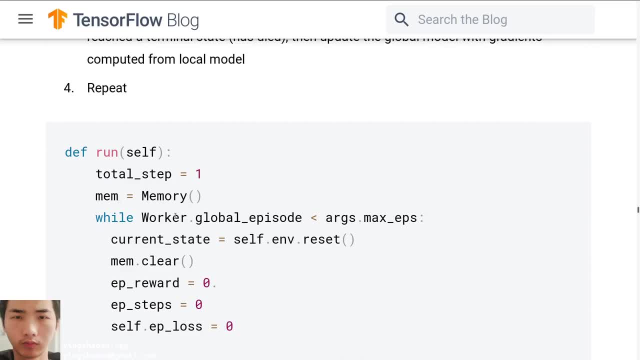 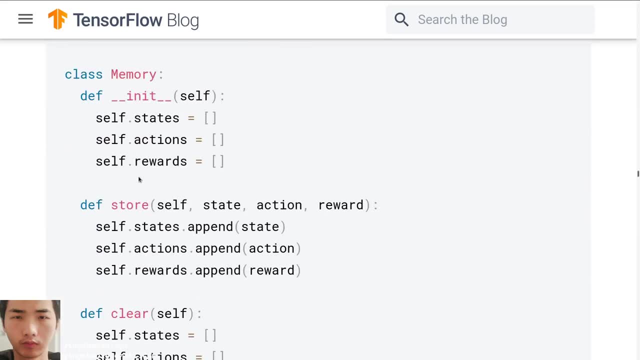 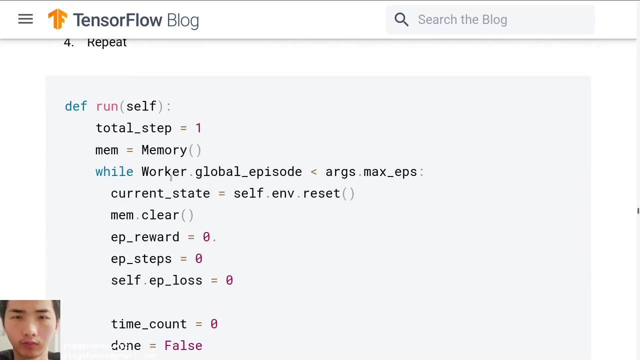 The mem equal to memory. Did you still remember the class that we defined, The memory class? It's just a way to manage the three last, While workerglobalEpisode less than the maxedEpisode With a current state equal to selfenvelopmentreset. 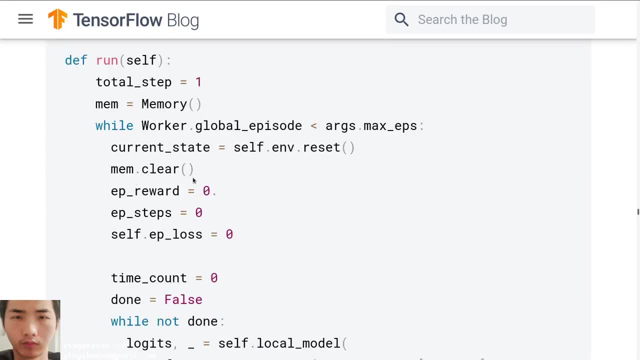 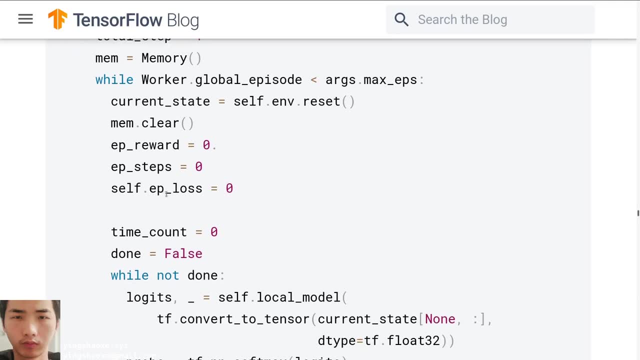 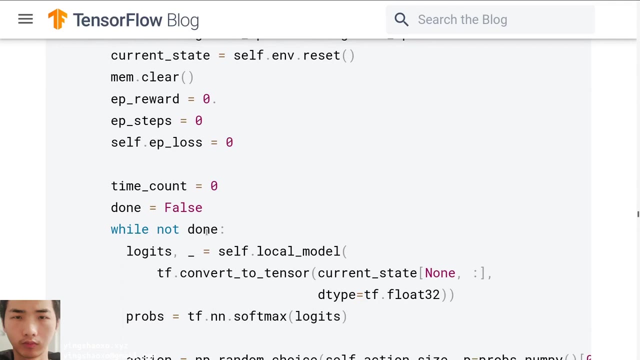 Memory Clear: Episode reward equal to zero. Episode steps equal to zero. The self Episode loss equal to zero. Time count equal to zero. Done equal to false. While Not done Will not died, Will not died, We say. 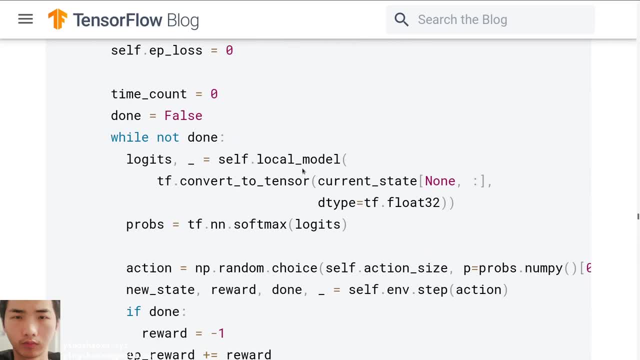 Logix equal to selflocalModel. We gave it a few parameters. We gave it a few parameters, I mean the current state- and then we calculate that logics and we want to know the biggest probability action. you know the largest probability of an action. 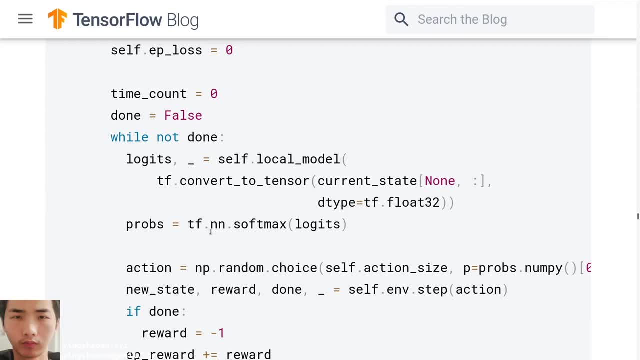 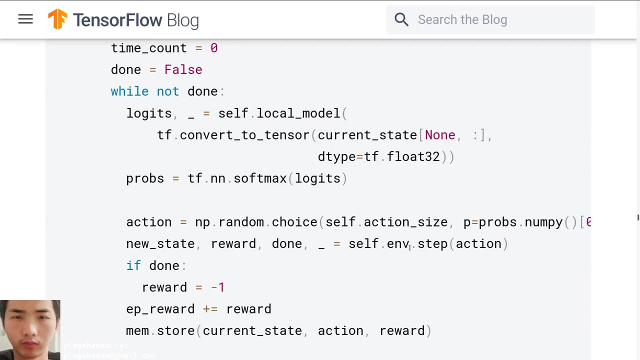 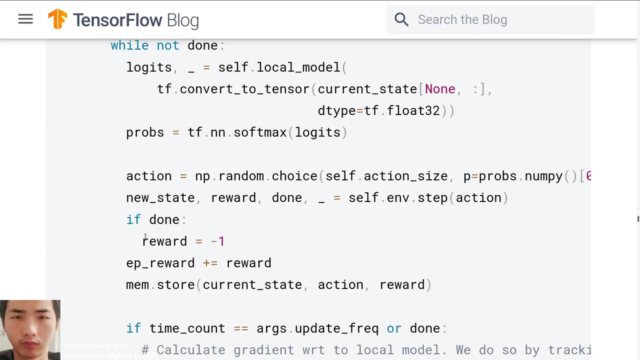 I mean what kind of action, what action we should take from this model? then we take an reading action and we give this action. you know, we take that action to the environment. if done, if it is died, if it's dead, we see the reward equal to negative one. 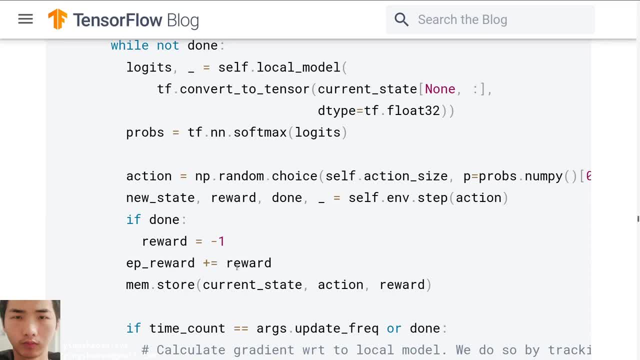 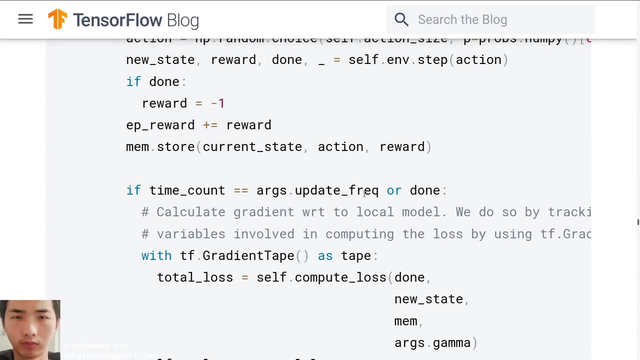 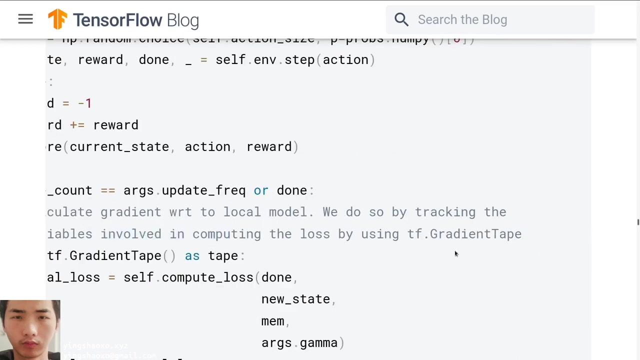 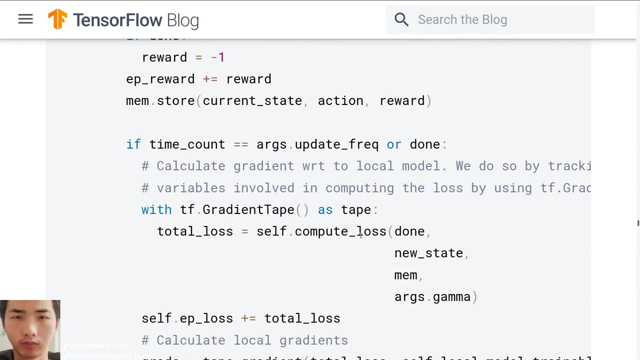 the absolute reward plus equal to negative reward, the memories we're going to store, the current state, the action and the reward, if time count, equal to the update frequency or done. we calculate the gradient with tfgradient tape as tape total loss equal to selfcompute loss done. 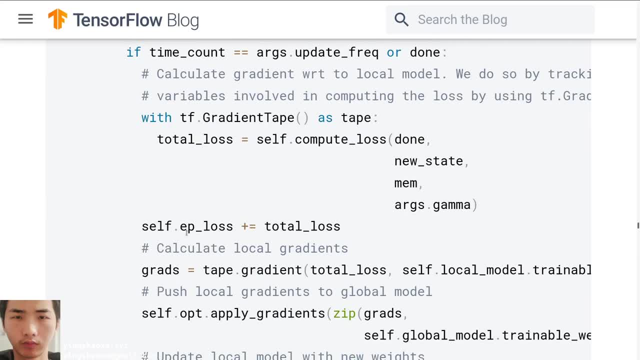 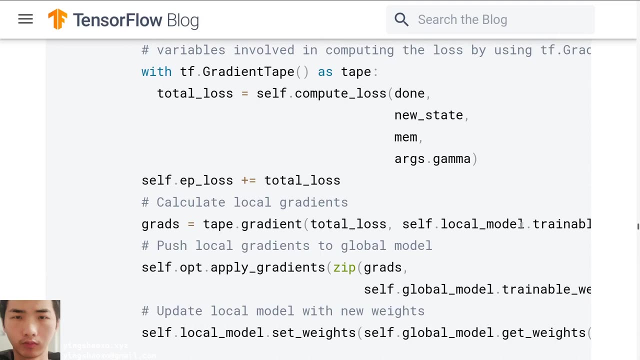 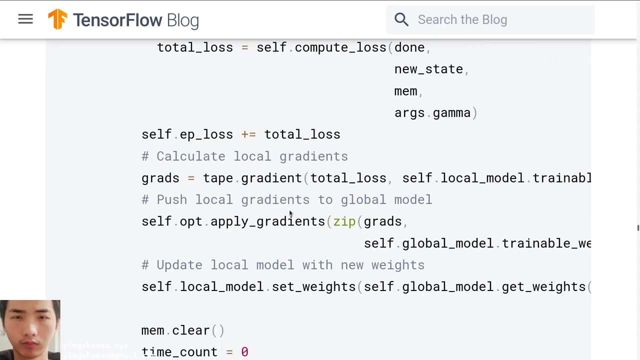 new state memory gamma selfperseverance loss plus equal to the total loss. we calculate the local gradients: gradients equal to typegradients. total loss: selflocal model that trainable push the local gradients to global selfoptimizer that apply gradients. Okay, here's the situation. 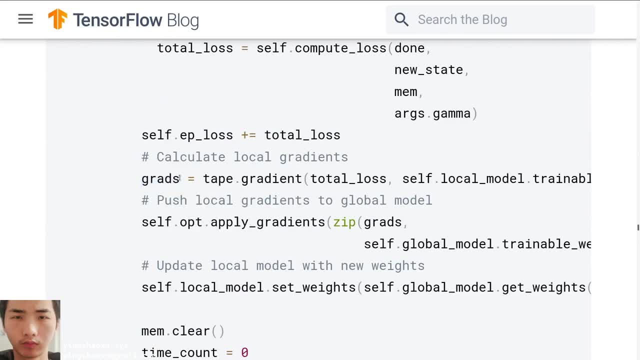 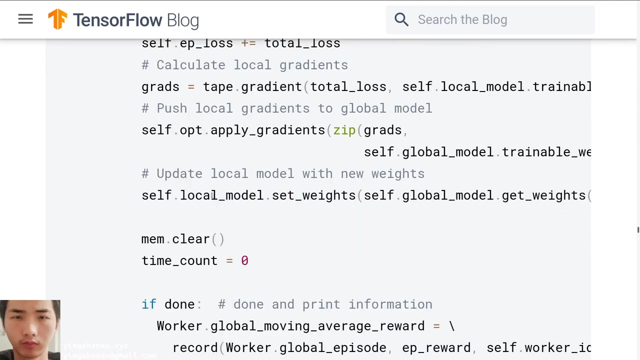 I mean the grades- here is the local grades and here is the global weights- And we just used an function, the optimizer applying gradients, to push the local gradients to global model. Then we update the local model with new weight. Save that local model that set weights. 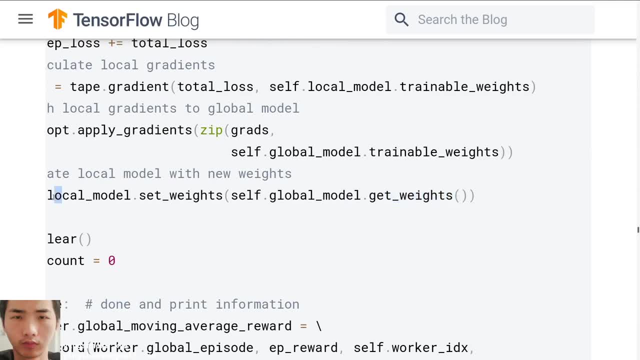 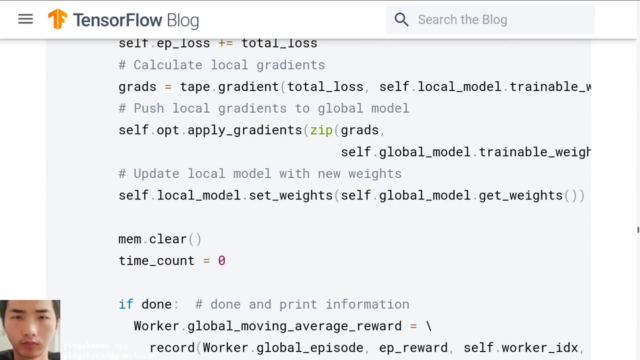 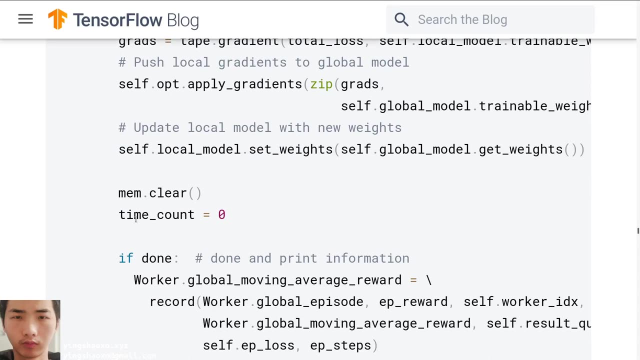 Save global model that get weights. Why? Why, he wanna use the global weights as the local model's weights. I have no idea about that. The memory clean, the time count equal to zero. If done, done and done, we get the open model. 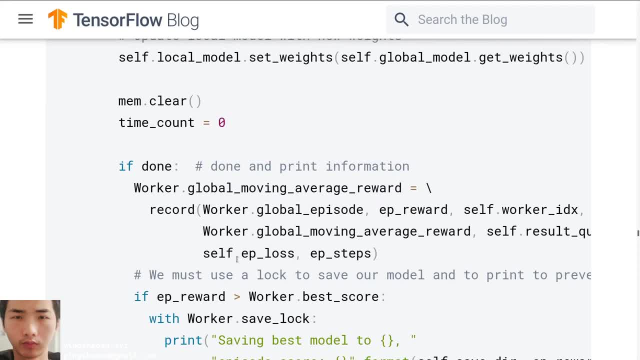 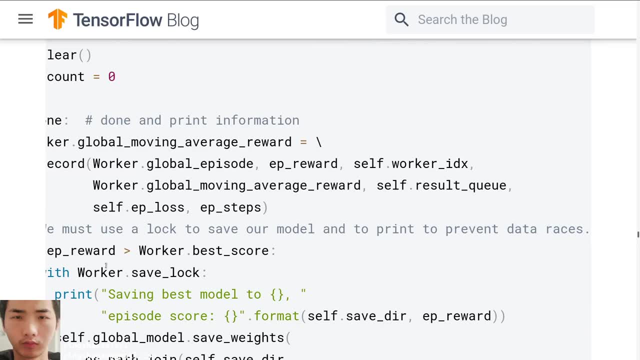 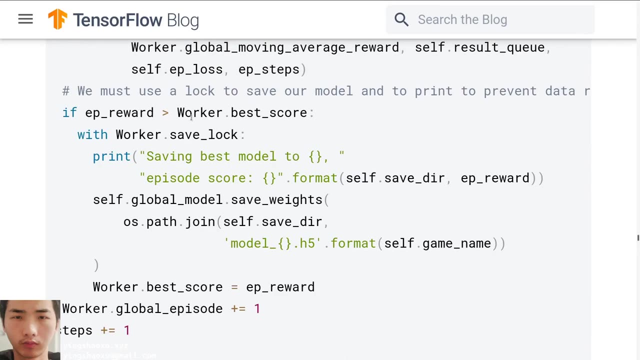 So let's look at the that protocol For local variableはい and to bring the information workerglobal empiezaverage reword equal to that, We must use a lock to save our model and to print to parent data data races. If eSeveralgretahrthankWorkerbas promotional. 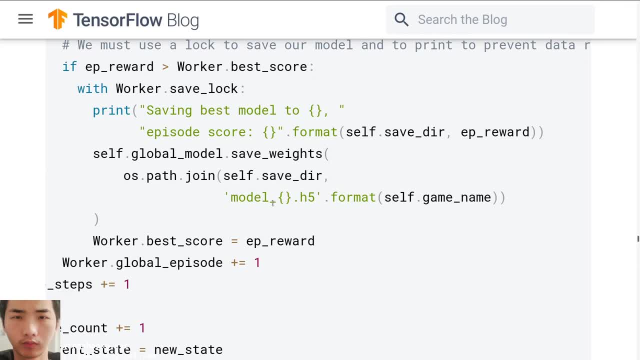 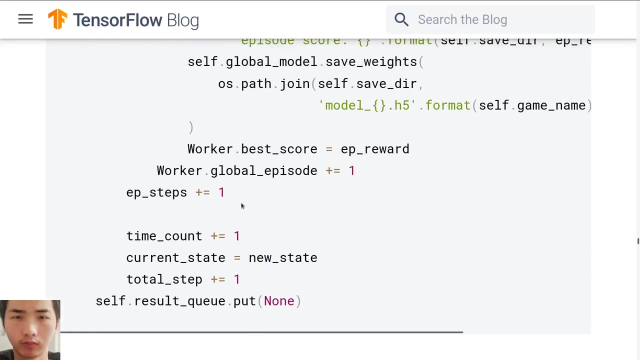 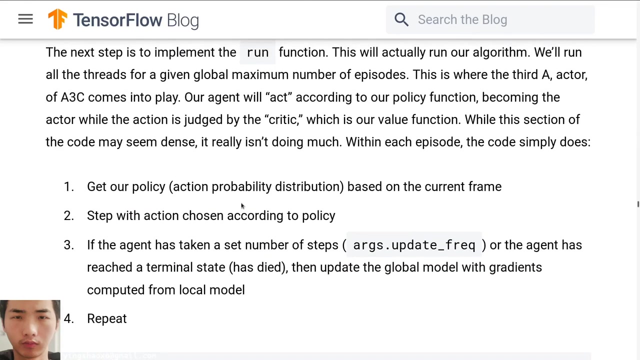 weights. Yeah, as for the model, here's an interesting fact about the model: The model is nothing but the weights, and the weights is nothing but matrices. Then we do this over and over again. Let's read the steps one more time. One get our policy or action probability distribution based on the. 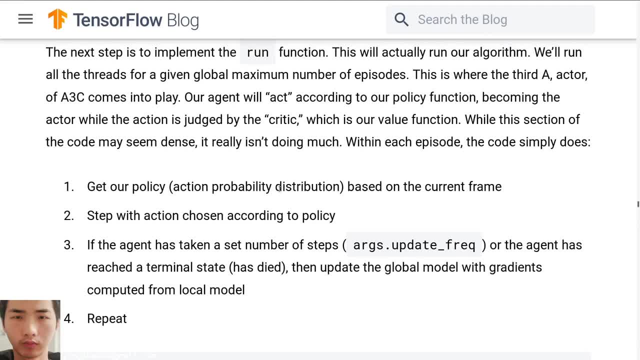 current frame The action probability distribution. the actual meaning of that is for each action we have, it has the probability to be the best action that we should take. so it's a table of action, probably probability to step with the action chosen according to the policy. yeah, we take that action to in the environments. 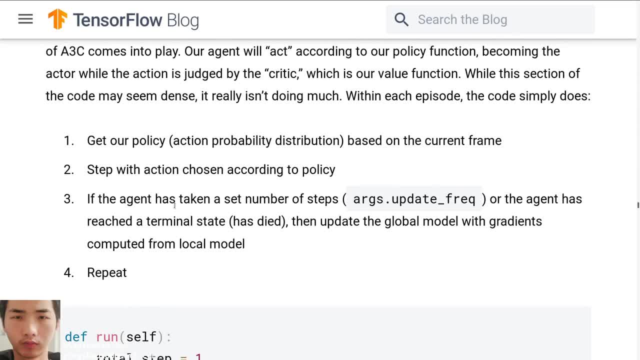 at the environments, if the agent has taken a set number of steps, or the agent has reached a terminal state. okay, here's a condition: if the, if the, if the agent has taken a number of steps, I mean how much steps we want the agent to run for one episode or for, for only when the agent execute that much of. 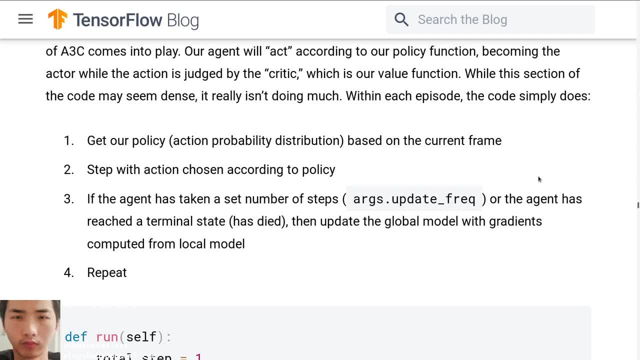 food actions. we update the data or the agent has that. if so, we update to the the global model by using the local agent models. data: when I see data, the data is nothing but but metrics, is but weights and all sorts of things. it's just like that. no, no big mystery. 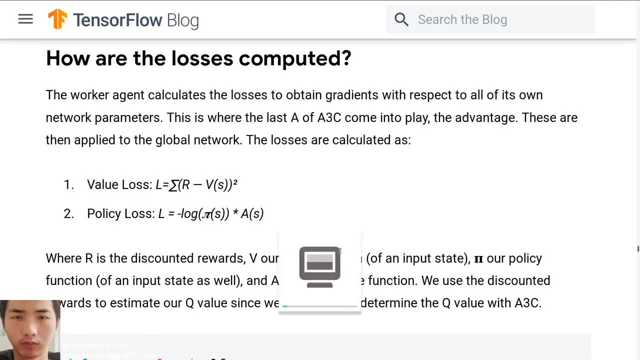 behind the scenes. that's how are the losses computed? the worker agent calculates the losses to obtain gradients with respect to call of its own network parameters. this is where the last a of a 3c come into play. the advantage in using this example is that of the 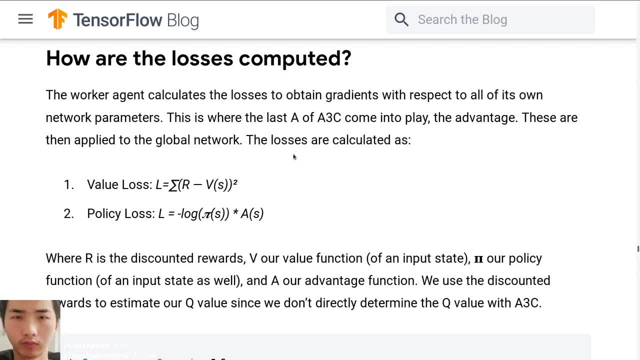 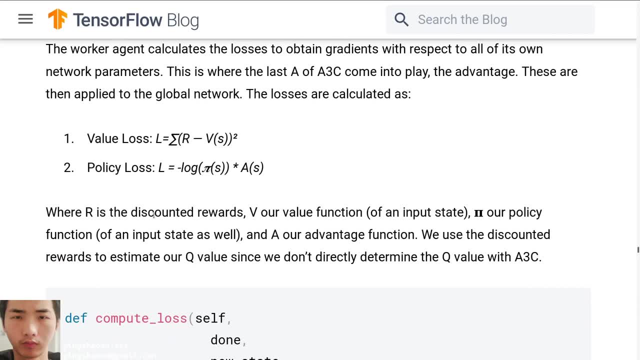 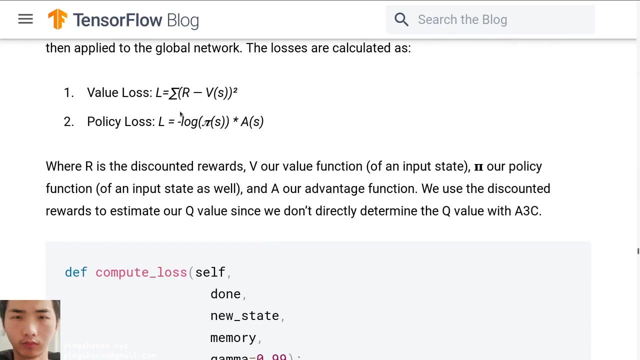 season here, so let us have a look at the B. these are then applied to the global network. the losses are calculated as this: it also takes the input state, And A is our advantage function. We use discounted rewards to estimate our Q value, since we don't directly determine the. 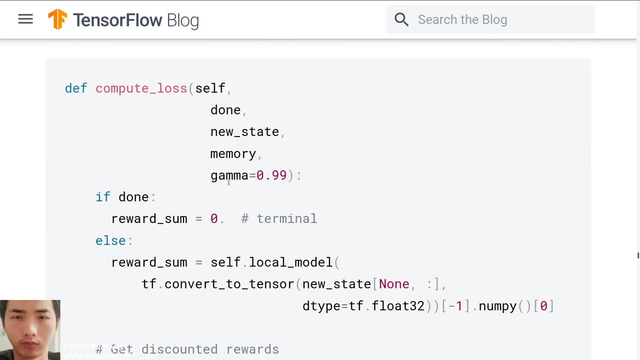 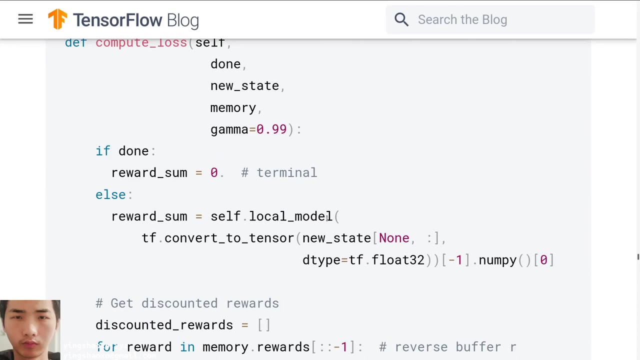 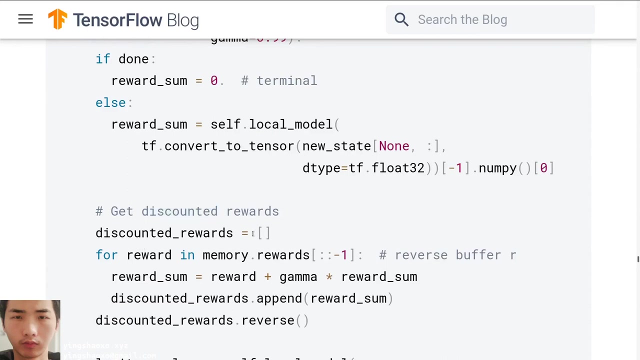 Q value with the A3C. Okay, here's the function computeLoss. If done, we say the reward sign equal to zero. Else we say reward sign equal to the local model. result: Get discounted rewards. Discounted rewards equal to an empty. 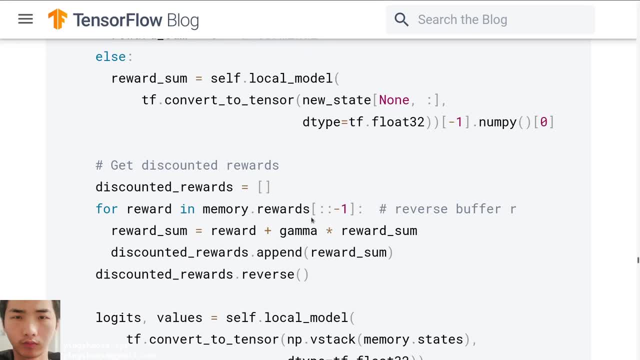 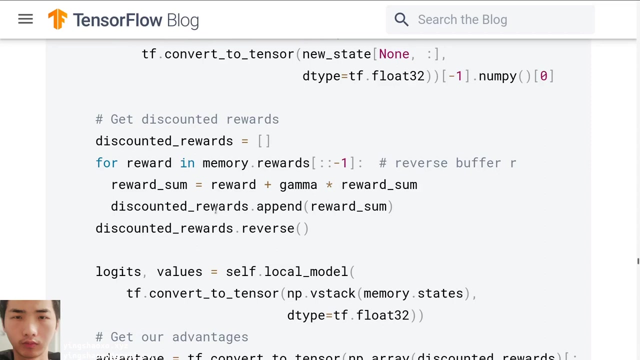 list For reward in memory that reward or we revert the buffer R. What this operation does is to meist the last, I guess the rewards matrix, or lest the The reward sign equal to reward plus gamma times the reward sign Discounted rewards. 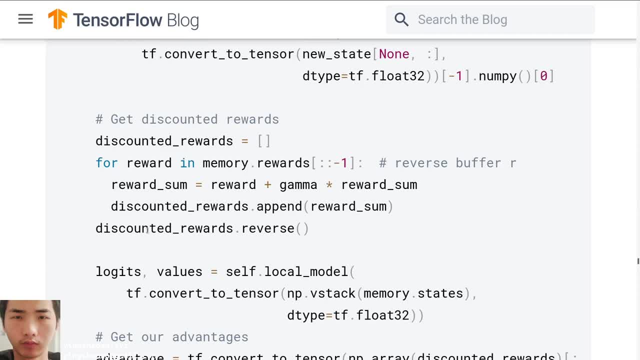 dot. append reward sign. Finally, we reverse the discounted rewards. dot. rewards: bar bar, bar bar. If we canonize this in there, Why would we call it discounted? It is because we will not use the original reward, but we will use the reward that changed. 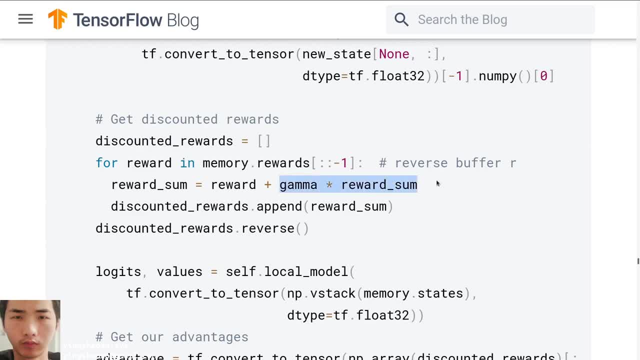 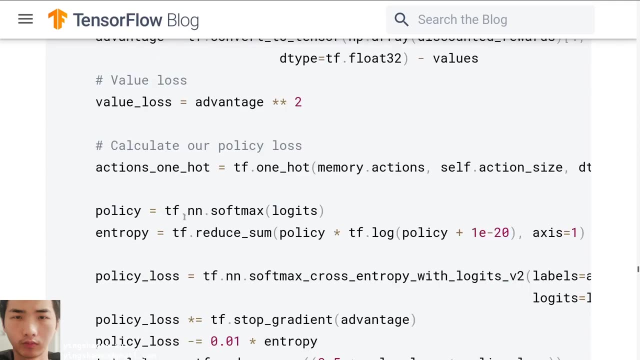 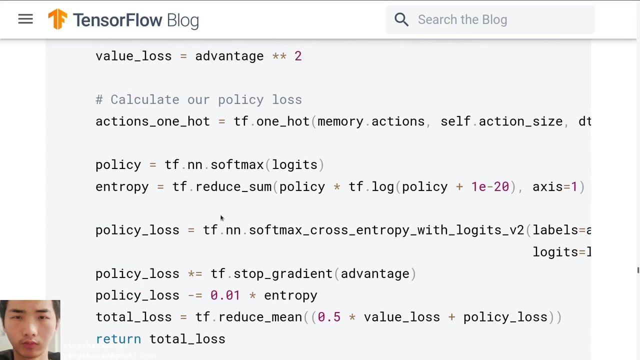 by this expression, gamma times the reward sum. The gamma is a superparameter or parameter for the machine learning project. As we could see here, the series of operations, it all relates to the tf. yeah, literally, I mean it relates to tf instead of keras. 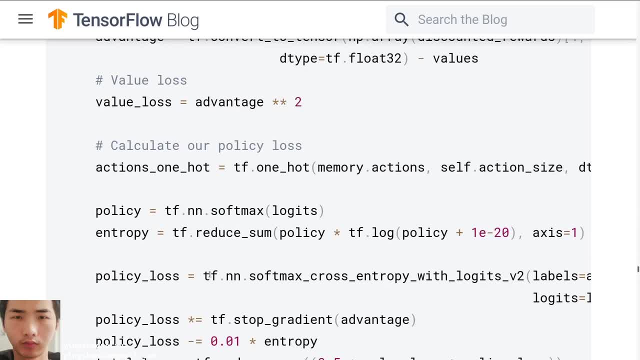 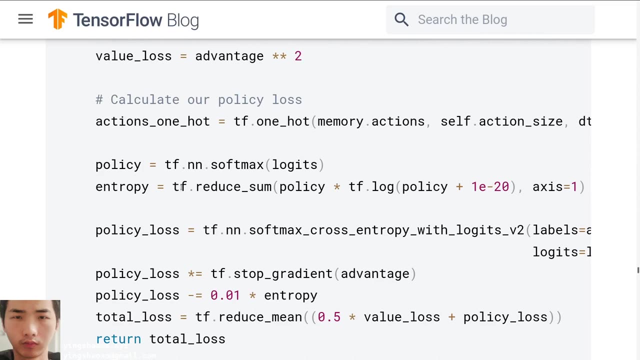 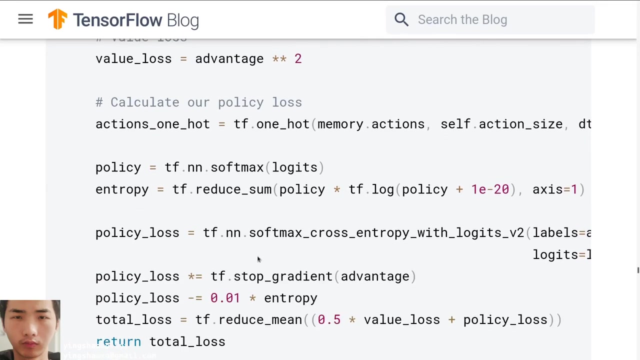 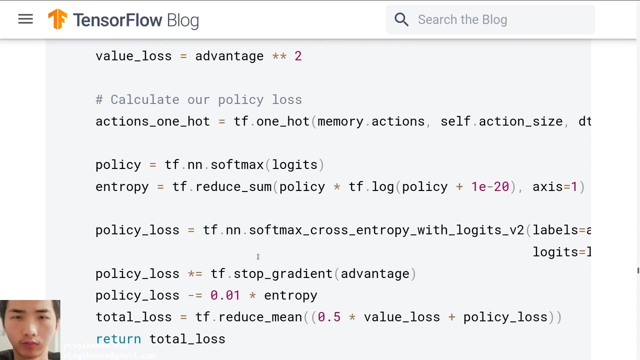 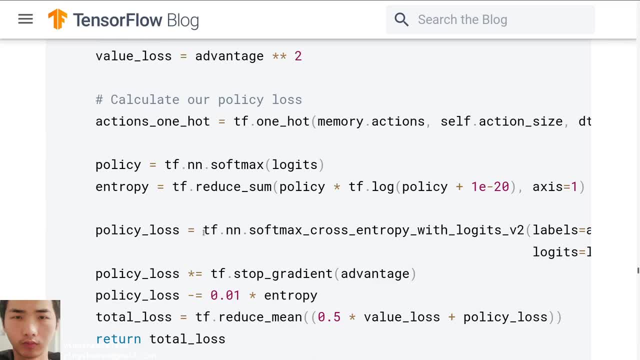 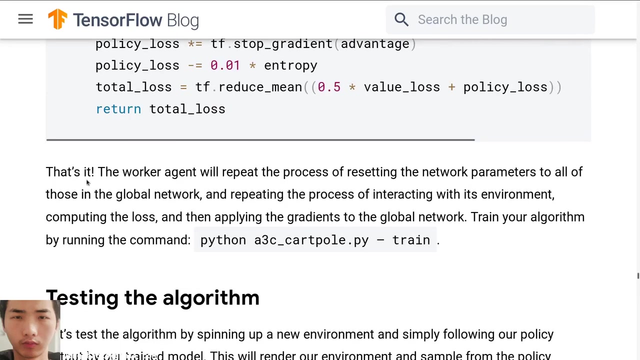 Well, the TensorFlow framework, it is nothing but a computing library. so it's a computing library. and what kind of computing library? Well, it's designed to process tensors or, to be specific, it is designed to process matrices. Yeah, that's all. 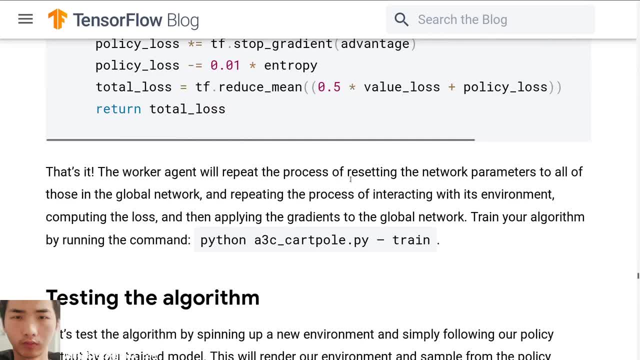 So that's it. The worker agent will repeat the process of resetting the network parameters to all of those in the global network and repeating the process of interacting with its environments, computing the loss and then applying the gradients to the global network. train your 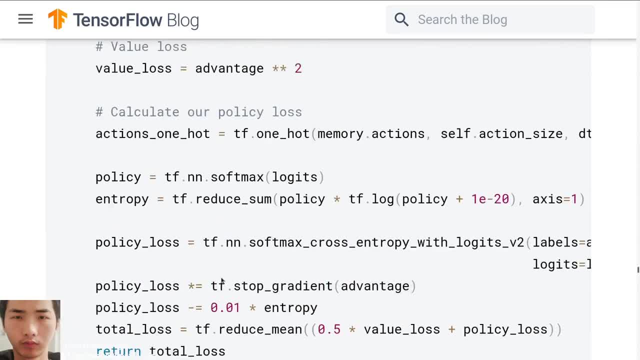 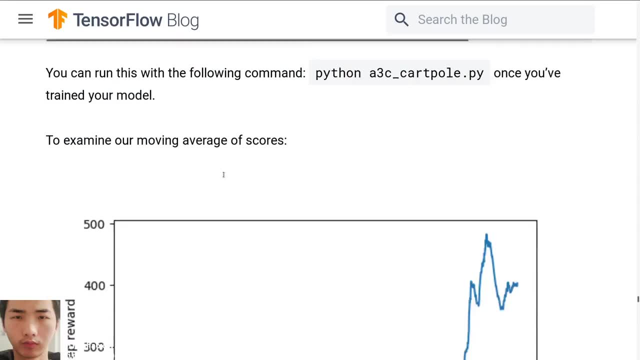 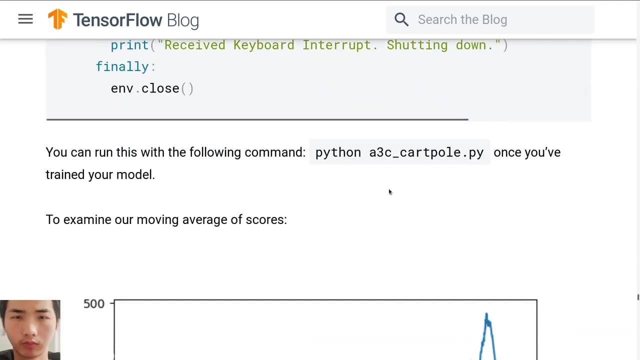 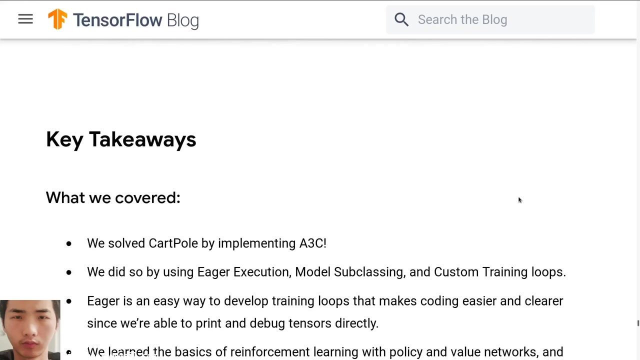 algorithm by running the command: Okay, I, We will not. Okay, We will not look into the testing section of that. It's not necessary, because it is tested by those people carefully and eventually it turns out: yeah, it works.